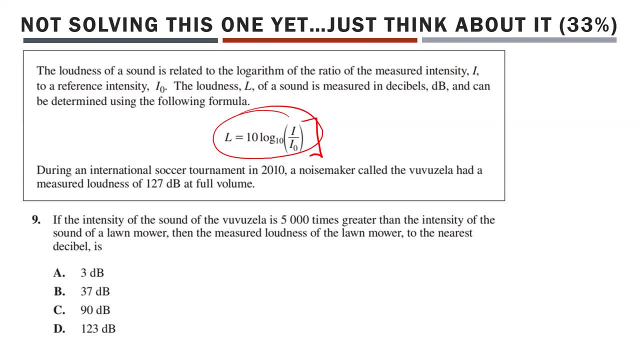 But there's another way to approach this, so we'll get into a little later on. If you want to pause the video here and actually give it a good read and think about it, you're more than welcome to. But aside from that, we're going to move on. we'll come back to this one later on. 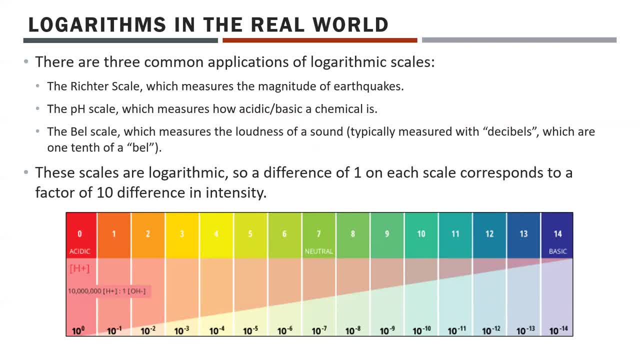 So logarithms in the real world. There are three common applications of logarithmic scales. there's- there's others than this, of course, but just three that you'll see more often in this course: The Richter scale, which measures the magnitude of earthquakes. The pH scale, which measures how acidic or basic a chemical is. you remember that from science nine, or chemistry, if you've taken it. 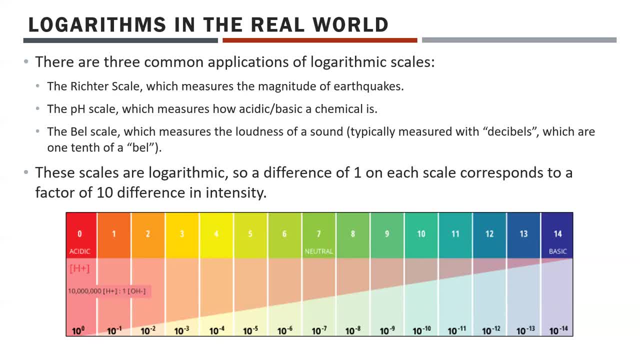 And then the bell scale, which actually measures the loudness of a sound. now, typically we don't use bells, we use decibels, which are one 10th of a bell. Same idea, though Now these scales are logarithmic, which means that a difference of one 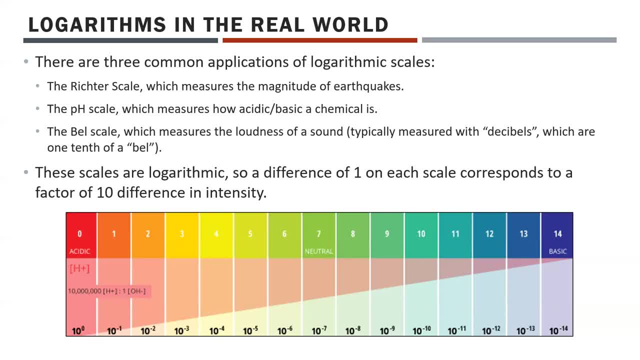 On each scale corresponds to a factor of 10 difference in intensity. So in other words, if you go up like- this is a pH scale, this whole rainbow looking thing right here- If you go up by one pH you're losing 10 times as much concentration of hydrogen ions in, you know, in your solution, right? 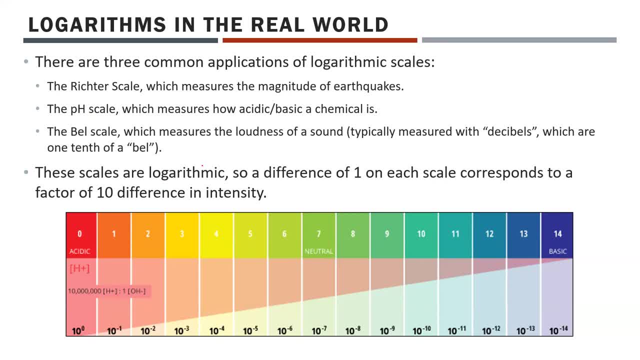 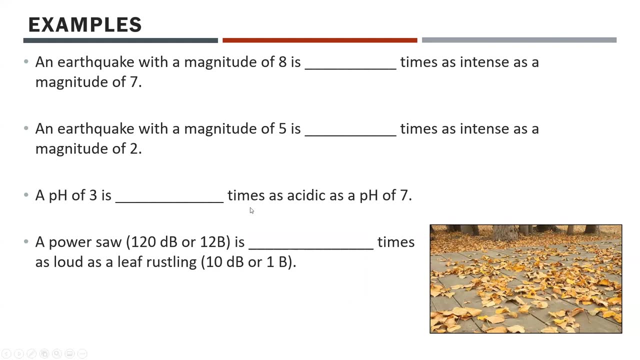 Same with the Richter scale. if you have a like a magnitude three earthquake versus a magnitude for earthquake, that magnitude for earthquake is 10 times More intense. That's what we deal with: logarithms, logarithmic scale Anyway. so for some examples here, an earthquake, once again with a magnitude of eight, is blank times as intense as a magnitude of seven. 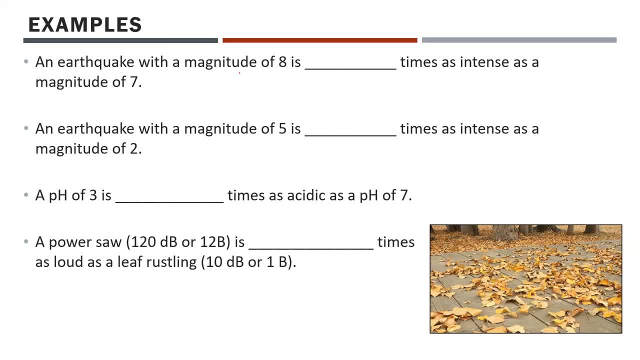 Well, since that's just one difference on this scale, That's a difference of 10 times more intense, Right? so the magnitude of 810 times more intense, the magnitude of seven? What about an earthquake with a magnitude of five? how does that compare to an earthquake with a magnitude of two? 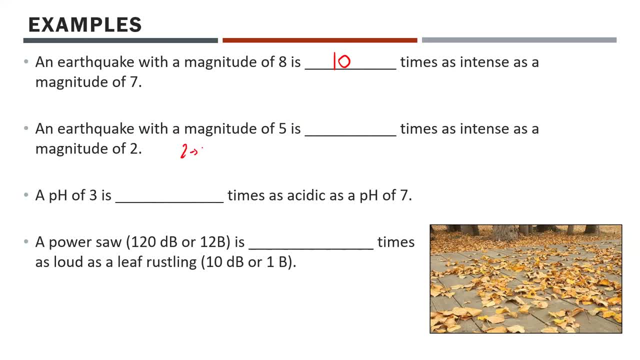 Well, let's put it this way: From two to three, That would be 10 times difference. three to four is another 10 times, and then four to five is yet another 10 times, but 10 times 10 times 10 without be 1000 times as intense, right? so they all kind of cascade onto each other, right? 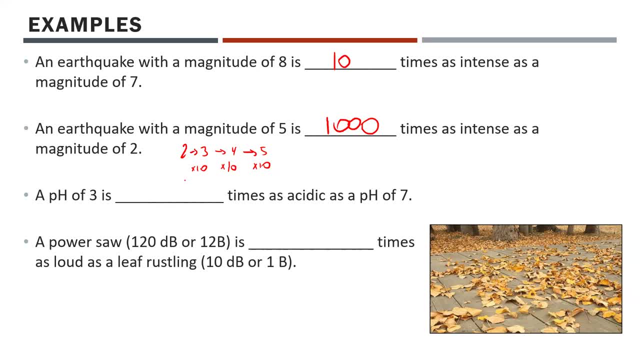 Next one: a pH of three is blank times acidic as a pH of seven. just a reminder: with pH, the lower your pH number, the more acidic you are, so so that that isn't backwards or anything: you, That is written correctly. Anyway, if we follow this back, seven to six would be 10.. 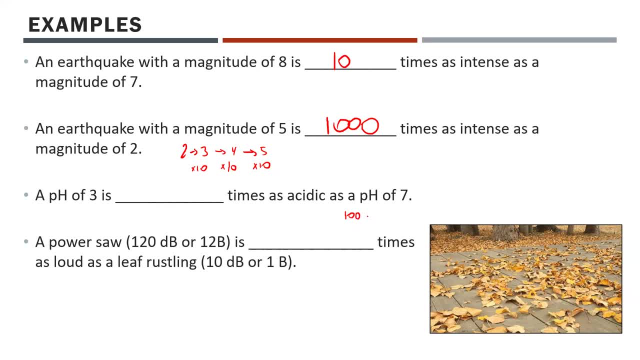 And then six to five would be 100,, five to four would be 1000, and therefore four to three we're at 10,000, right? so I just added a zero for each one of the differences I was counting back from seven to three. 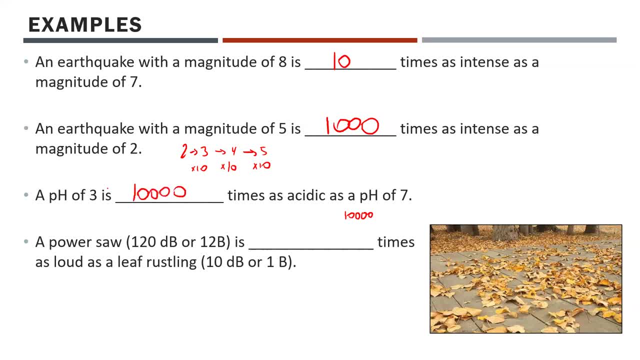 That was what I was just doing there, so 10,000 would be the answer. their pH or three is 10,000 times as acidic as a pH of seven. The last one here a power saw which is 120 decibels or 20.. 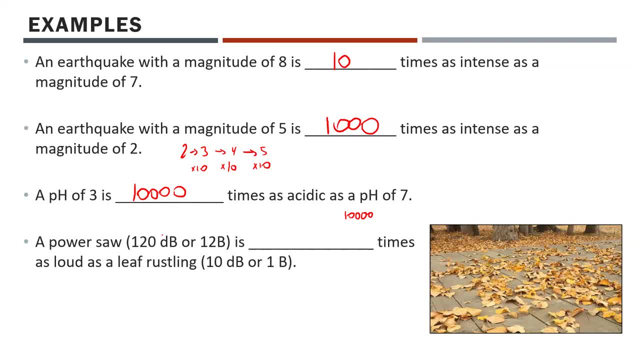 That's right, That's right. So that's 12 bells, if you prefer, because remember, 10 decibels, as one bell is blank times as loud as leaf rustling, which is only 10 decibels, or in other words, one bell. 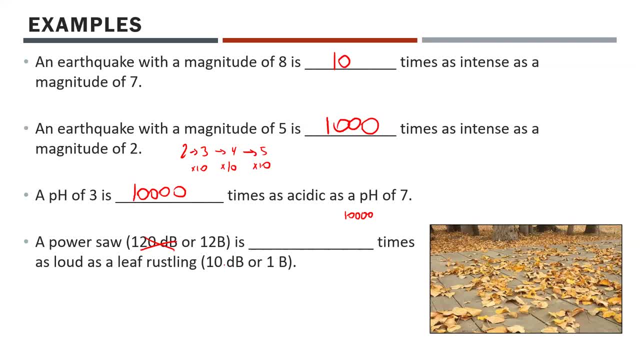 Now decibels. of course, that's used for communicating, but in terms of actually doing calculations, I'd recommend you ignore it. Look at the difference between 12 bells and one bell. If we were to count backwards there, watch this or 12. Maybe I'll go the other way. so it's talking about how much louder it is. Let's start at one. we'll go one to. two is 10 times. 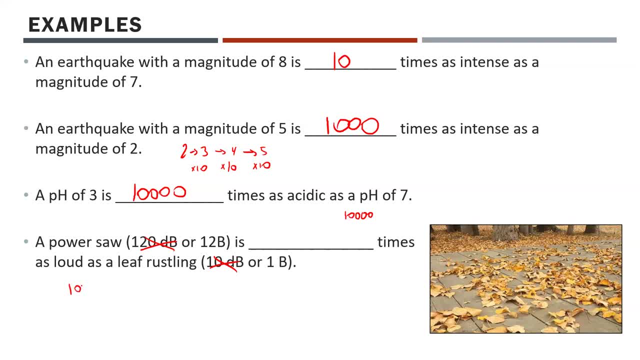 More intense. Two to three we're at 100, and then four, and then five, and then six, seven, eight, nine, 10,, 11, 12. Number right there. so if I break this apart, We're interested to see. that's 100 billion times as loud as a leaf rustling wouldn't. wouldn't seem like that, like it's kind of hard to quantify that, but the math checks out here right. 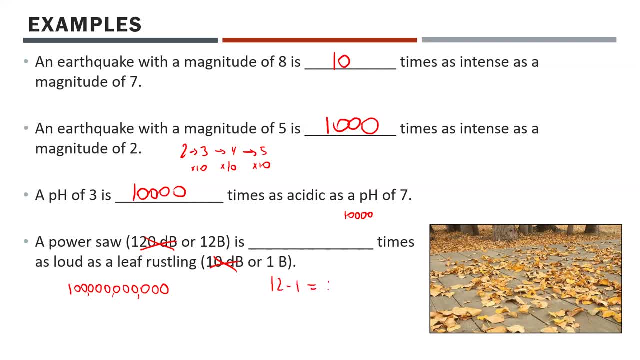 Another way you could thought of that is 12 minus one. the difference between that is 11.. Notice how many zeros there are in this number. Count the zeros up there. If you count the zeros up, they'd be 11 zeros. We'll use that actually. so, once again, 100 billion times as loud as a leaf rustling. 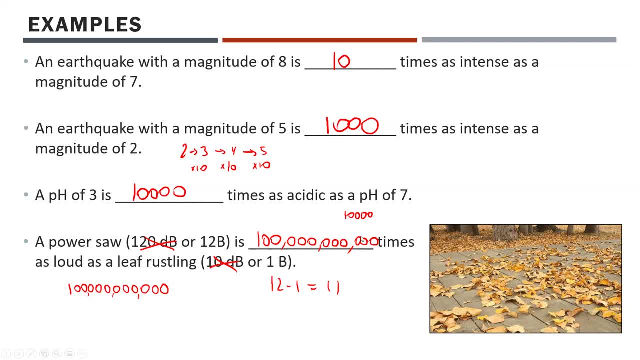 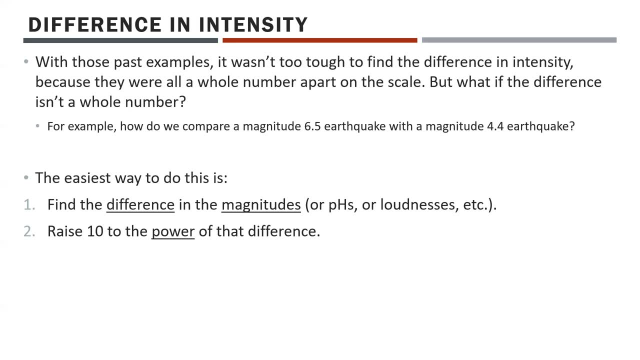 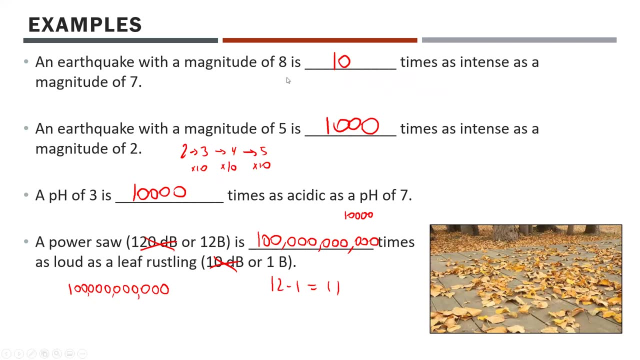 Again sounds mind blowing, but it it checks out, believe me. Anyway. so difference in intensity: with those past examples it wasn't too tough to find the difference in intensity because they were all a whole number apart on the scale. So in other words, if you noticed, like like just going back here, eight to seven, that's a whole number apart, it's just one apart. five to two, whole number apart. 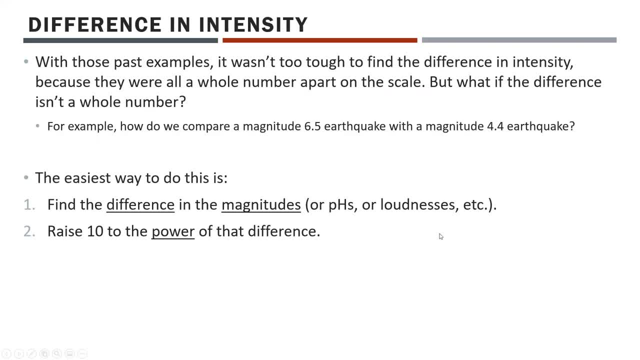 It's just one apart, Five to two, whole number apart. So there's a three difference. right, you get the idea. But what if the difference isn't a whole number? So, for example, how do we compare the magnitude 6.5 earthquake with a magnitude 4.4 earthquake? 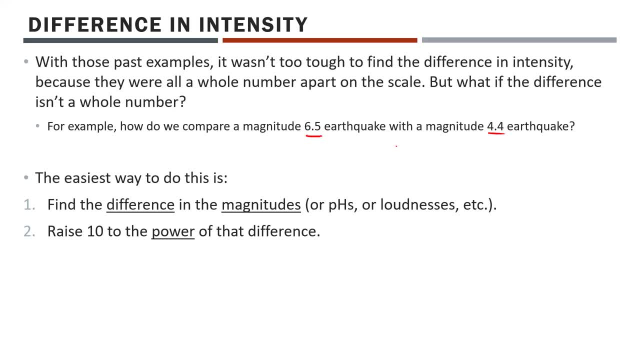 You know that's going to be like 2.1 difference there. that's not a whole number. we can't just like add, you know, 2.1 zeros onto something. doesn't make sense like that, right. But here's the easiest way to do this, And I was alluding earlier when we looked at that diploma question. This is usually my go to strategy, no matter what kind of question I'm dealing with, with an application of a logarithm. 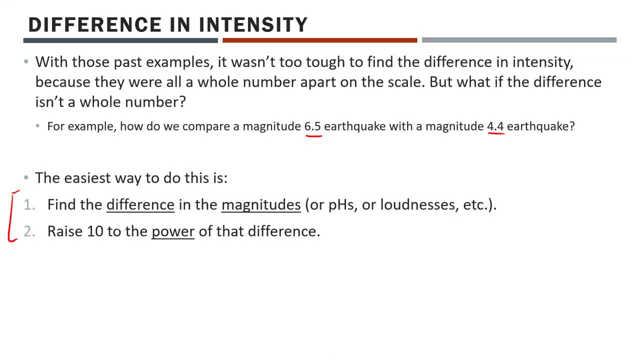 This is how I go about it. Step one: find the difference in the magnitude. so where the pH is or loudness is whatever you got, I'll just call them magnitudes for now. So find the difference. difference means subtraction, So in this case would be 6.5 minus 4.4, that's a difference of 2.1.. 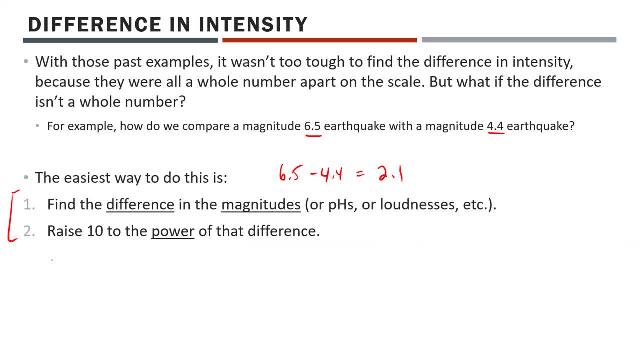 Alright, so I find that first Step two, this is our last step. it's just that quick already. raise 10 to the power of that difference, So in other words, 10 in this case to the power, To the power of 2.1.. 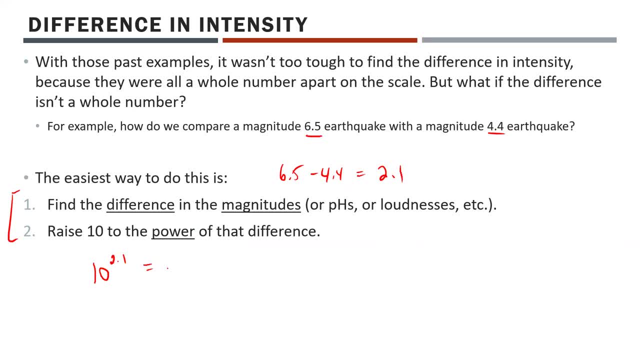 Now I don't know what that is off the top of my head. you're gonna have to use a calculator for that. so 10 to the power of 2.1.. I'm just going around to the nearest whole number. It's about 126, 126 times more intense. So we knew if it had a difference of two, like 6.5 to 4.5, that's a difference of two. 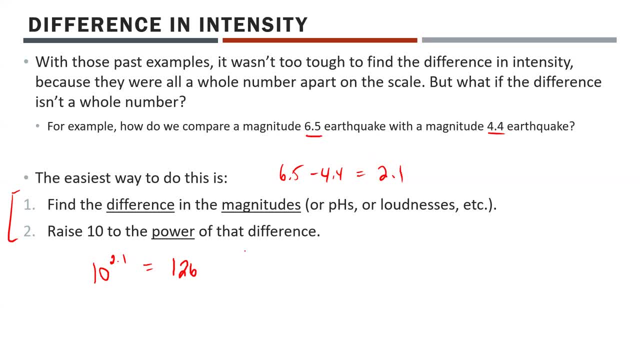 Well, that'd be 10 times 10, so 100 times different. 2.1 adds quite a bit more, right, so it's 126 times more intense. That's how we deal with it, right? so step one: Find the difference. Step to raise 10 to the power of that difference. 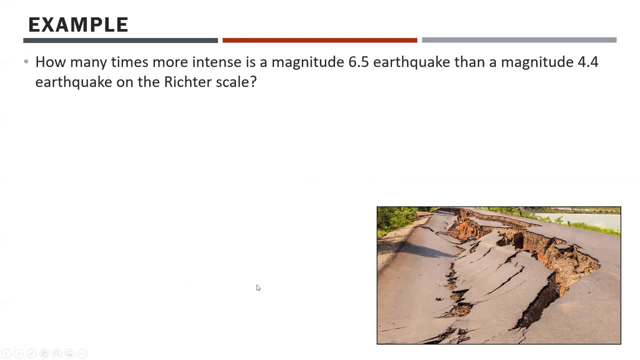 Oh, look at that, we already did it. next question here already. so that work I just did. I totally forgot that. I threw that in there. magnitude 6.5, magnitude 4.4. you know what, forget it. I'll just do it one more time: 6.5 minus 4.4 equals 2.1, 10 to the power that. 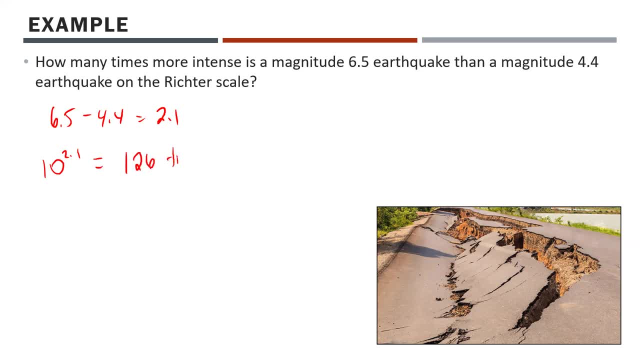 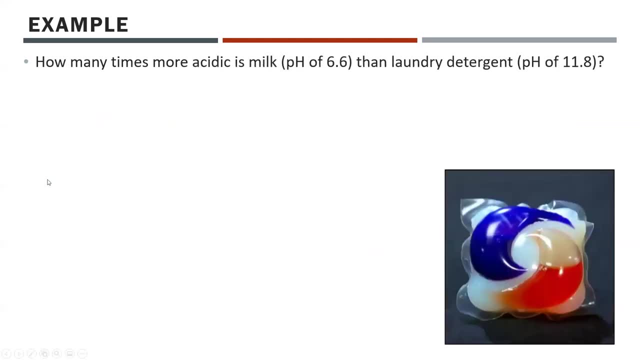 10 to the power 2.1, that gave us roughly 126 times right, 126 times more intense. That's all. Next one: how many times more acidic is milk, which has a pH of 6.6, then laundry detergent, which has a pH of 11.8.. 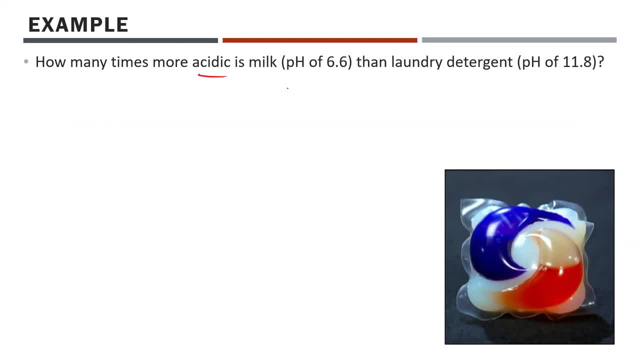 Remember, acidic is lower on the pH scale, so the question still makes sense. So we're looking at how many times more acidic it is. just take the difference between those two numbers, so we'll go 11.8 minus 6.6.. Just typing that in just so I don't get mental math wrong. here it's 5.2. 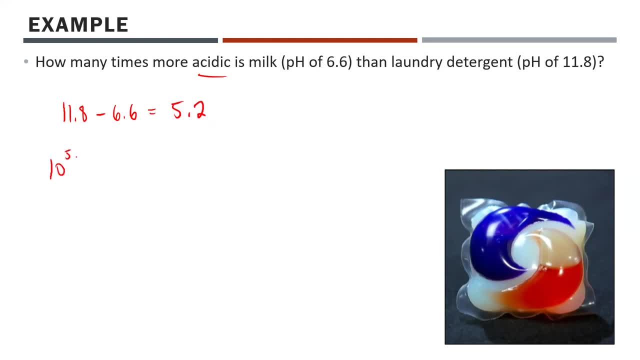 There we go And then raise 10 to the power of that, so 10 to the power of 5.2.. Remember that in your calculator as well. give me a second: 10 to the power of 5.2. just rounded to the nearest whole number is 158,489.. 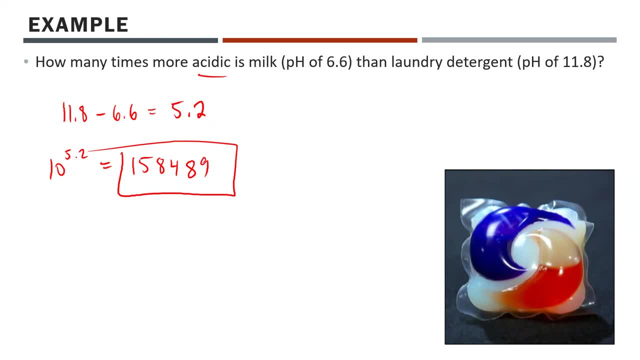 There it is right. super quick, super clean, super simple. right, just find the difference between your intent or your magnitudes and then go 10 to the power. that difference that gives you your difference in intensity. so 158,489 times more acidic. 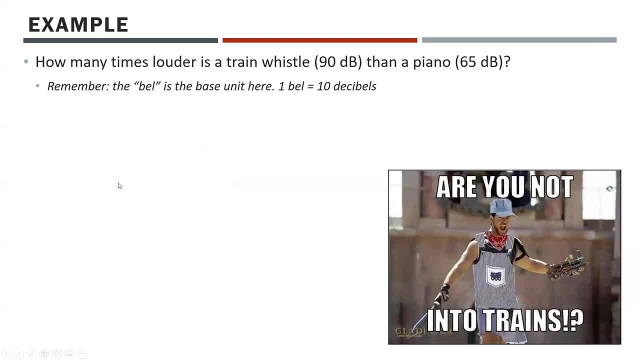 neat, right. moving on, What about this one? how many times louder is a train whistle, which is 90 decibels? That actually sounds too low. a train was only being 90 decimals. But anyway, I won't, I won't argue it. let's say: train whistle 90 decibels, that a piano which is 65 decibels, And just remember, the bell is the base unit here. one bell is 10 decibels. 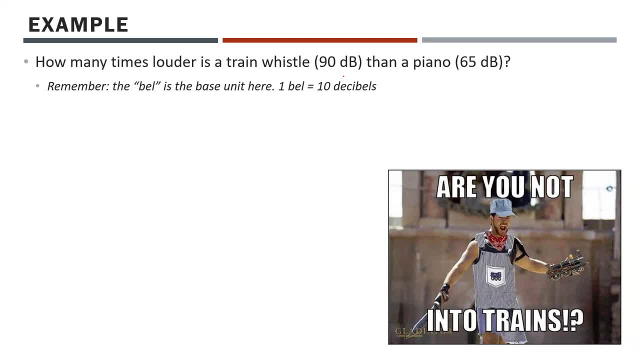 So to go about doing this, anytime I see decibels, I'm going to change this into bells right away. so one bell is 10 decibels. So here we go, Here we go decibels. so 90 decibels, that's nine bells. 65 decibels, will that be 6.5 bells? right decibels. 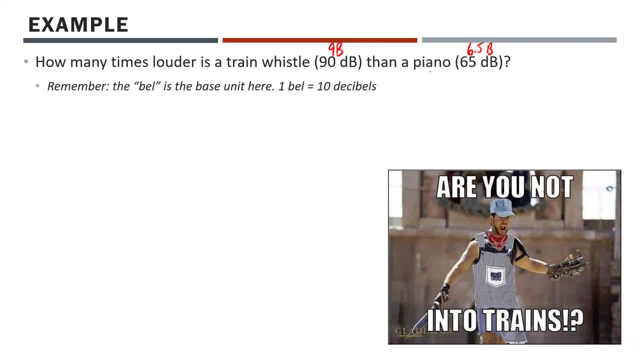 are better for communicating. that's just what we use. but bells are the actual, real unit. that's what we need to use here. um, anyway. so strategy here, as always, to find how much more loud that is, just find the difference. so nine minus 6.5, that is of course 2.5, and then just go 10 to the power. 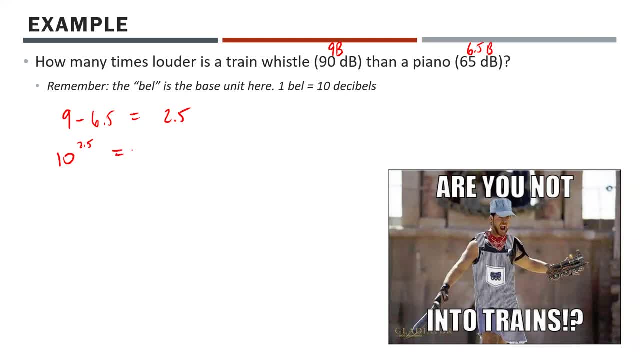 of that. so 10 to the power 2.5, that is going to equal, just to the nearest whole number, 316 times. so according to this question, a train whistle is 316 times louder than a piano. but in all honesty i think that's way too low. i think a train whistle is probably probably more than 130. 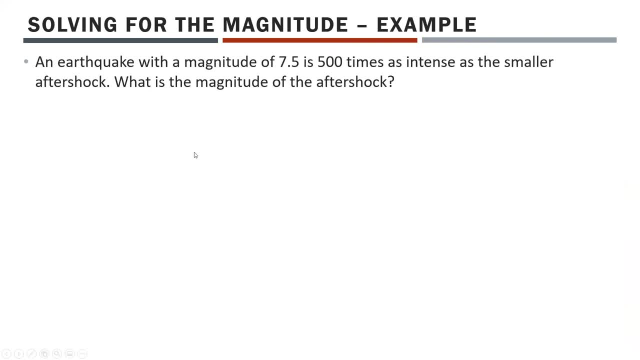 decibels it's. it's very loud, but anyway, i'm not going to argue with this, all right. so this question is going to stir things up a little bit. we're going to move um kind of backwards here. so in this question we're going to move um kind of backwards here. so in this question we're going to 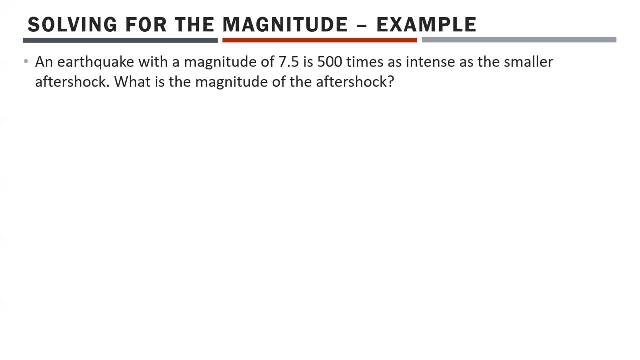 say, an earthquake with a magnitude of 7.5 is 500 times as intense as the smaller aftershock. what is the magnitude of the aftershock? well, in previous questions we would take the difference between your magnitudes, so 7.5 minus the magnitude of the aftershock. that would give us what we raise. 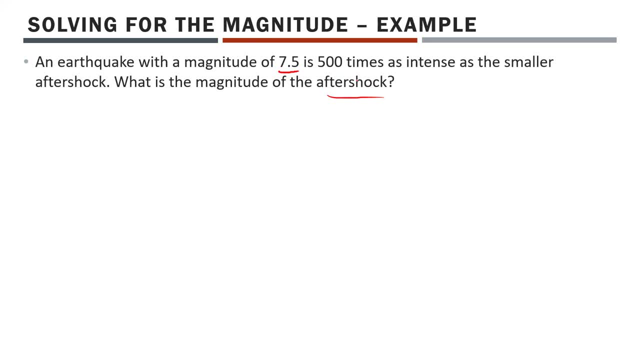 to power to get to 500. in this case, we're just going to have to work backwards. bear with me on. here's how my brain works. with this one, 500 is like that's the difference in intensity, that's how many times more intense it is right. so i know. 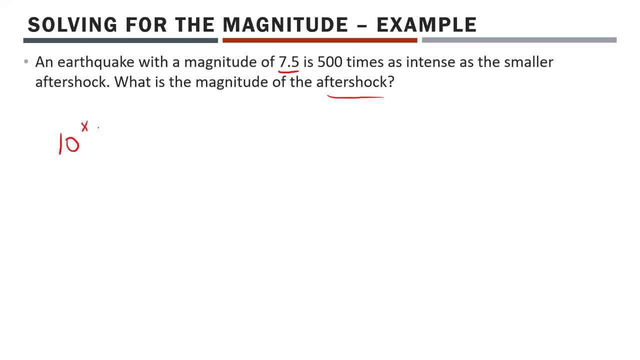 10 to the power of something i'm just going to call it x. 10 to the power of x equals 500, right now that x represents the difference between our magnitudes, right? so usually we would go 7.5 minus whatever and then go 10 to the power of whatever that was, and that would give us our 500, but we 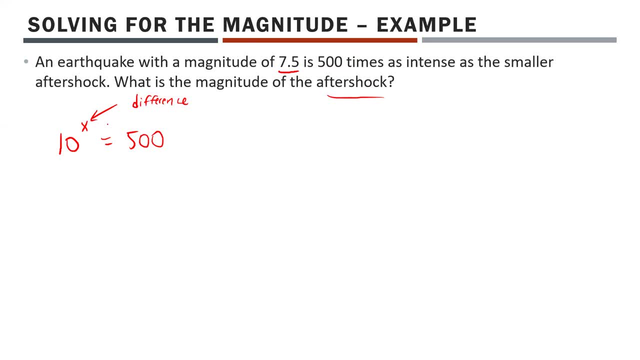 have to work backwards here. so just keep in mind: x is going to represent our difference in this case. now, if only there was some way we could solve for x here. like, are we going to have to guess and check this? i'm just kidding, of course we're not going to have to guess and check this. this is an 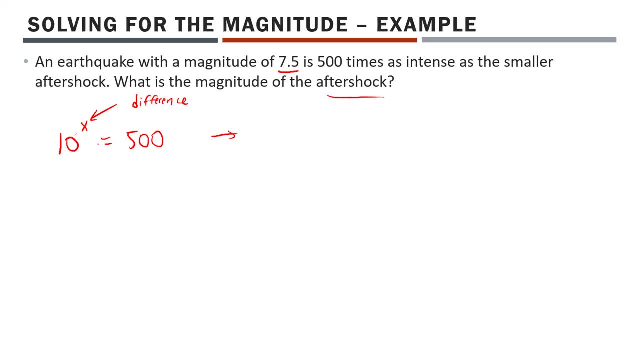 exponential function where x is the unknown up in the, up in the power. there we can just use logarithms to solve this, just as we've been doing earlier in this unit. uh, to do logarithms here, just do the old switcheroo. the base becomes the base of the log. so this is going to be log base 10. 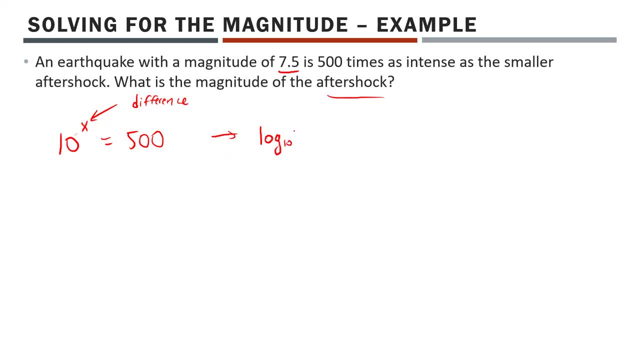 you don't even have to write base 10 because if you just write log you'll assume that. but i'll be kind here, i'll write log base 10. the answer is what goes into the log. so 5 goes into the log and then the answer: the log is the thing that was your old exponent, so that's. 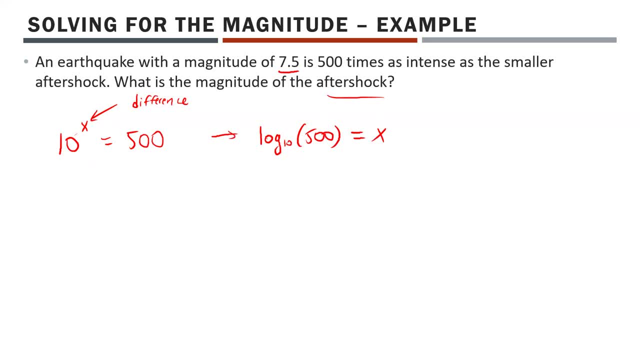 going to equal x. type that in your calculator real quick: log base 10 of 500. you just press log of 500 because remember, just basic log is log 10. uh, what i got for x when i did that, i got x equals. uh, you know what? i'll just take the two decimal places. that's actually going to round up. 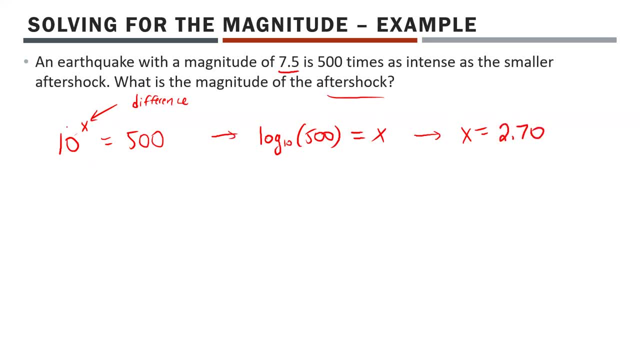 to 2.70. now remember what i said earlier. x represents the difference, so in other words, 7.5 minus something equals 2.70. maybe i'll write that out: 7.5 minus something equals 2.70. well, to find this, of course. 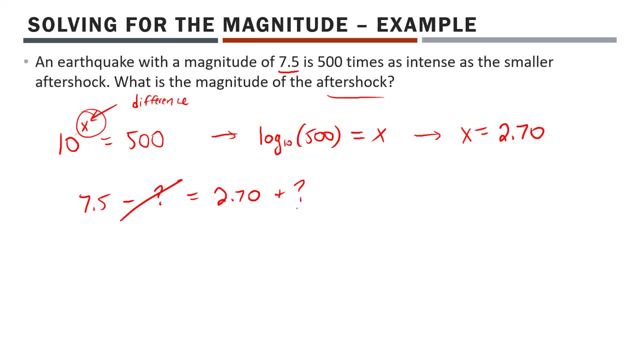 we just need to add the something on both sides- there it is- plus something, and then subtract away your 2.70. long story short: 7.5 minus 2.70, this is going to give us our unknown equals 4.8. that right there, that 4.8, that is the magnitude of your aftershock, right? 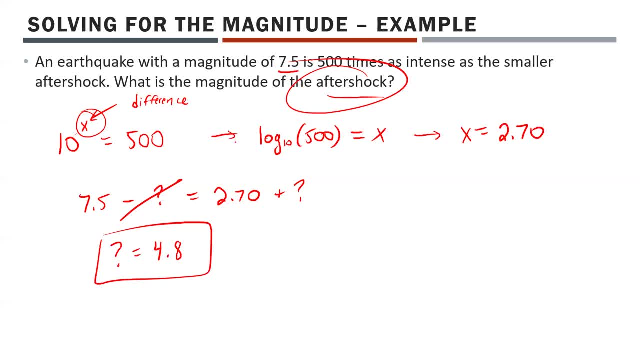 if you don't believe me, you can always work backwards, find the difference between those two and then go 10 to the power of that difference. you're going to get something pretty darn close to 500, right, we round it here, so it won't be perfect, but it'll be pretty darn close. 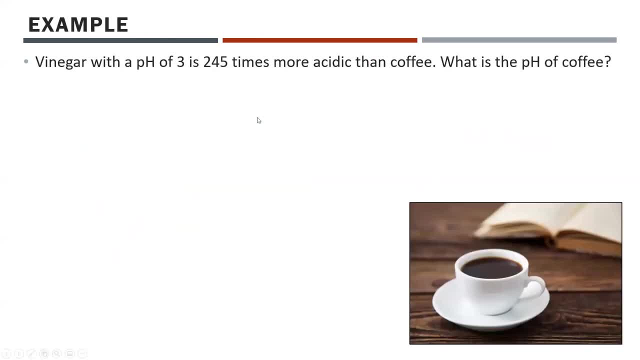 anyway, let's keep rolling. next, next example here: vinegar with a ph of 3 is 245 times more acidic than coffee. what is the ph of coffee? okay, so since vinegar is more acidic, uh, and ph is kind of backwards, we're a little bit more acidic than coffee. we're going to get 3.5 times more acidic than coffee. 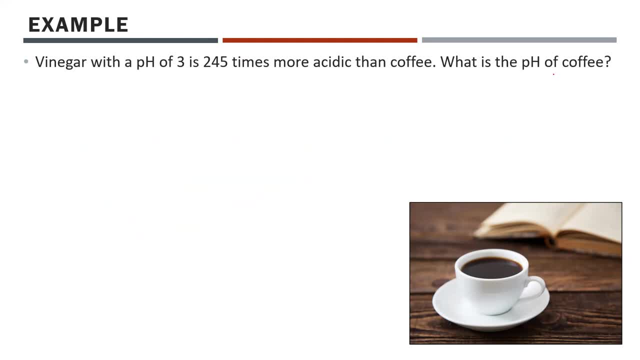 lower pH is a more acidic pH. We know that the pH of coffee is going to be some number bigger than three, right? So, in other words, it's going to be something greater than three, right? Just keep that in the back of your mind. Otherwise, this question is done the exact same way as the other. 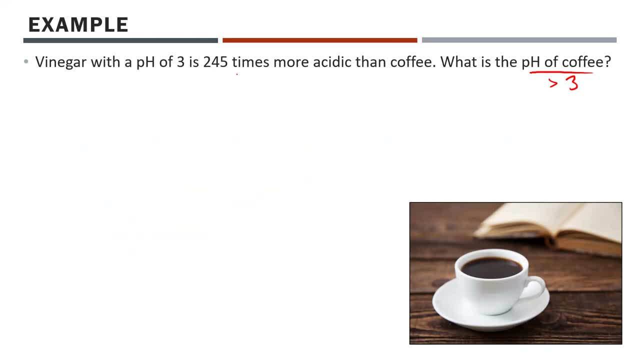 one. Let's take that difference in intensity, like how many times greater it is, and let's make that equal to 10 to the power of X. So 10 to the power of X. so this X, representing once again your difference, 10 to the power of X, equals 245.. Well, just like before, we need to use logarithms. 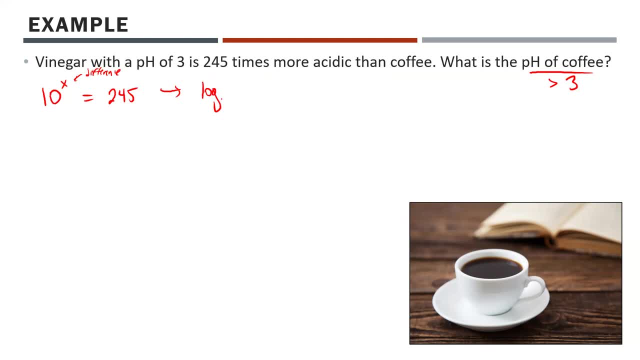 to solve this. So log base of the log is going to be the base of the exponent here. so log base 10 of the answer goes into the log. so of 245 equals our X. Give me a second here: log base 10 of 245,. 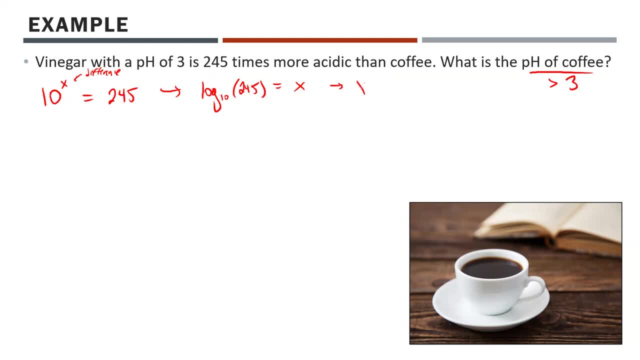 that's going to give me. I'll just round to two decimal places again. X equals 2.39.. So 2.39.. That's our difference. Now, remember, our answer is going to be for coffee. Coffee, is you know? 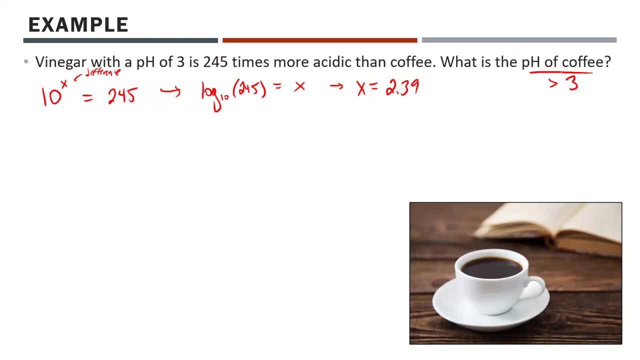 we already were told vinegar is more acidic than coffee, so coffee has to have a bigger than three pH. So let's put it this way: Let's call question mark the pH of coffee. The pH of coffee is question mark minus the pH of vinegar. so minus three equals 2.39,. right, We just have to add. 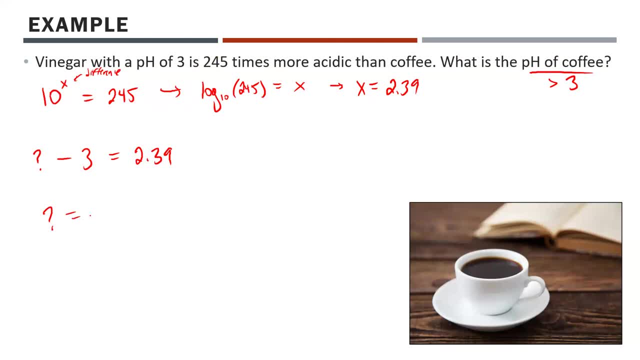 three on both sides. That's all we're going to do here. Question mark: the pH of coffee equals 5.39.. It doesn't say what to round to, so you know what. two decimal places is great. You could have done just one if you wanted to like. 5.4 would have. 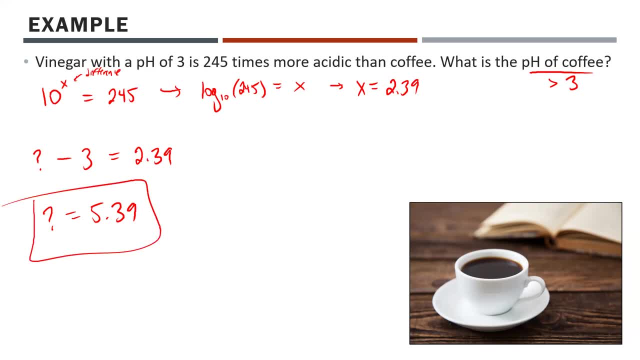 worked just fine. Whatever you do, though, that is going to be the pH of coffee, And again, if you don't believe me, you can always work backwards right. 5.39 minus three, that'll give you 2.39.. 10 to the power of 2.39 is 245.. We know how many times more intense it is. 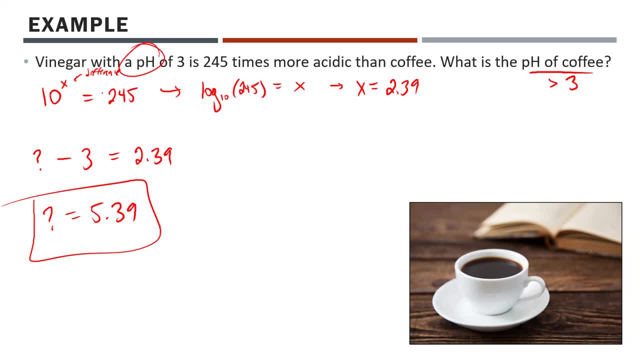 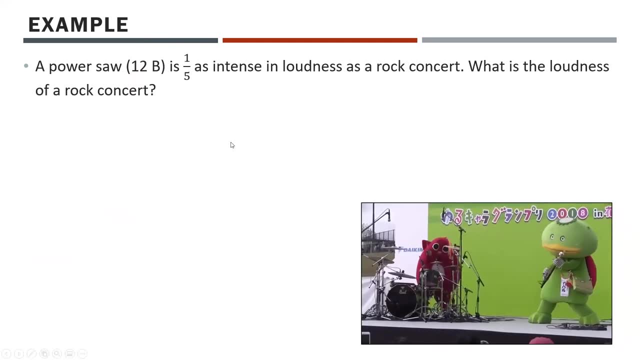 You just have to know. with pH, the scale again is backwards. The lower the pH, the more acidic that liquid is. That's basically all we're looking at. All right, here's another one, Once again with a power saw. I don't know what the interest is with power saws in. this is. 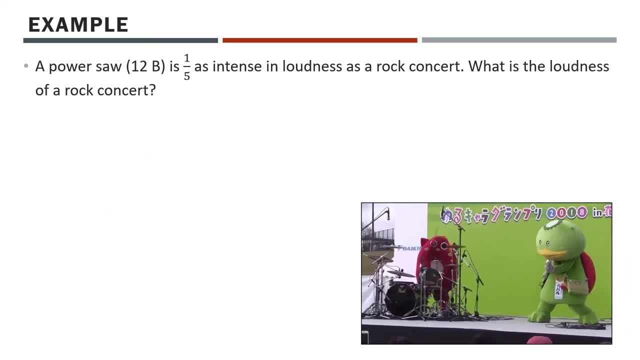 but it is what it is. So a power saw which is 12 bells is one-fifth as intense in loudness as a rock concert. What is the loudness of a rock concert? Okay, so this one's kind of like. 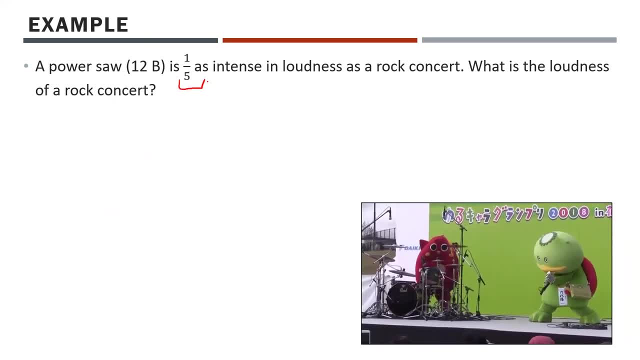 the last one, Notice it's one-fifth as intense. That tells us it's going to be like the power saw is going to be a lower number than the rock concert, So the rock concert is going to be greater than 12 bells. That might be important to note. However, 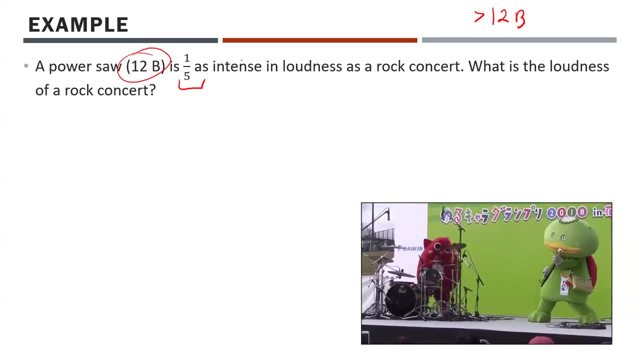 notice how small this number is here, right, One-fifth as intense- What I would almost assume. since we're going to have a one-fifth here as our difference in intensity, I'm going to actually assume that we're doing this a bit backwards and we're going to go the 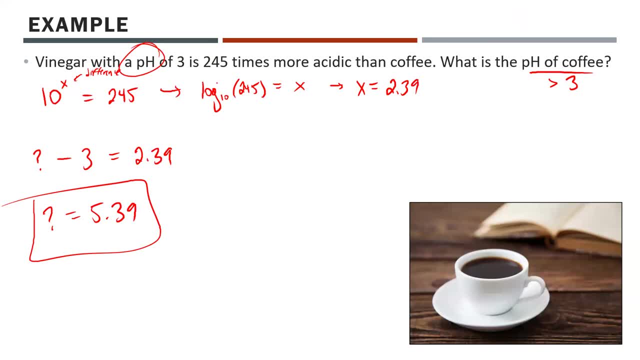 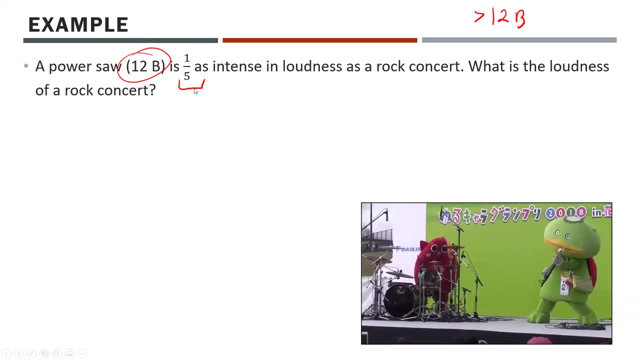 power saw minus the bigger number. Notice in all the other previous questions we did, we always went like the bigger number minus the smaller number, but that gave us a number that was, you know, relatively large. This number here is just one-fifth. If you don't believe me on this, 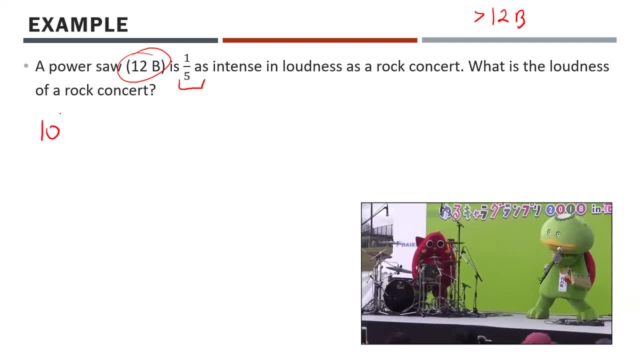 one watch what's going to happen, Just from the previous questions. here we're going to go 10 to the power. of x equals our magnitude or, sorry, our intensity difference here. So our intensity difference is one-fifth. Also, just like previous questions we've done, here we're going to change. 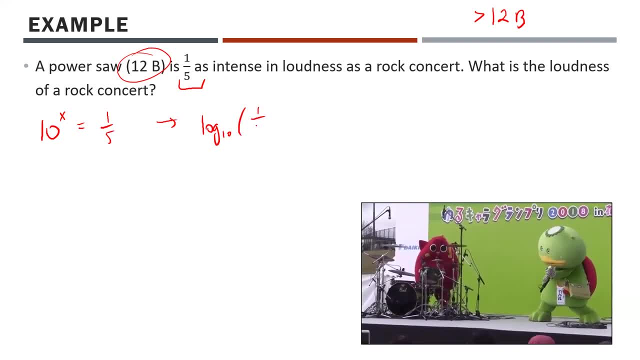 this into a log. So log base 10 of our answer, which is 1 over 5, equals x. If you throw that in your calculator log of 1 over 5, you're actually going to get a very strange number. for x, You're going to get x equals. 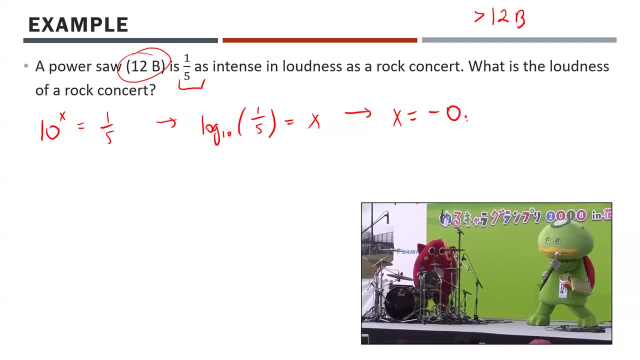 negative 0 point again, rounding just to two decimal places: negative 0.70.. Very strange number there, Like a really really really strange number there. It's so weird to have a negative as our difference right, Because that's what x is Remember. 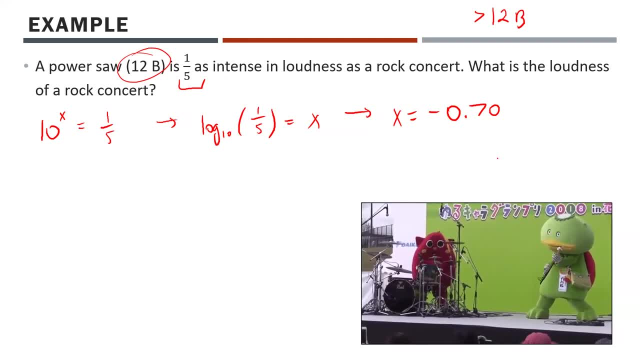 x is our difference. The only way we can have a negative difference is if the smaller number was written first, Like, for example: if you have like 4 minus 7, that'll give you negative 3, right. The only way- I don't know what's with my 3s lately- That's a negative 3, right. There we go. 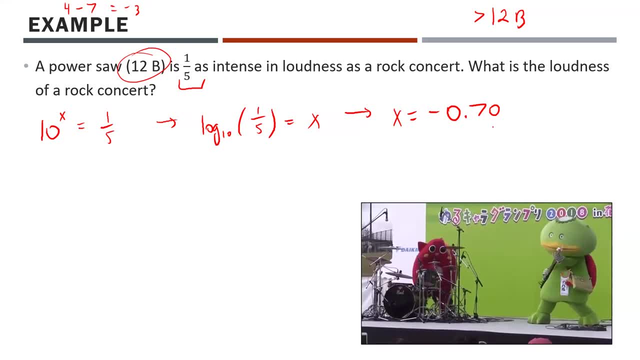 Jeez, Louise. Anyway. so 4 minus 7 is negative 3.. The only way you're going to get a negative difference is if you had a smaller initial number. Well, we know the power saw is not quite as loud as a rock concert. We know the rock concert has to be greater than 12 bells. The long story short. 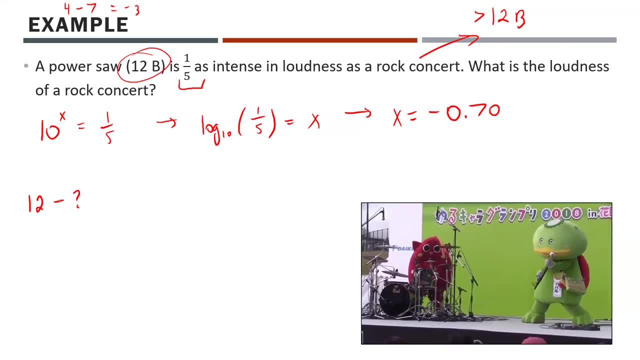 when I write this up now I'm going to say this is 12 minus something. smaller number minus bigger number equals negative 0.70.. That's about as true as it gets. So if you have a smaller number, tricky as they get, They really try to slip you up with that sometimes. Just be mindful of what it. 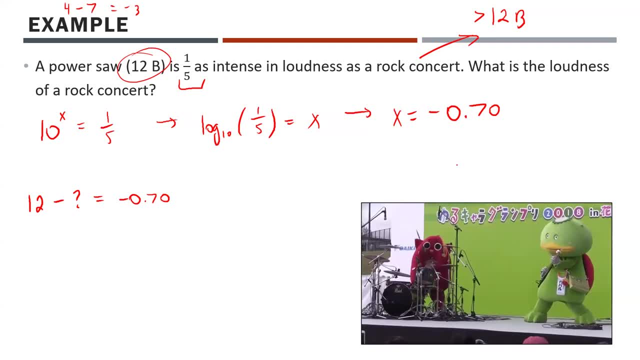 means to have a negative difference. You have to have your smaller number first. It's just a logic thing, right, Anyway? so since we're looking for this, we're trying to find the question mark. I think the easiest way to do this would be to add the question mark on both sides And then to get. 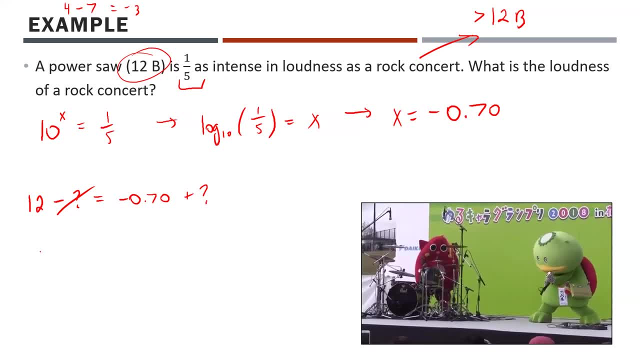 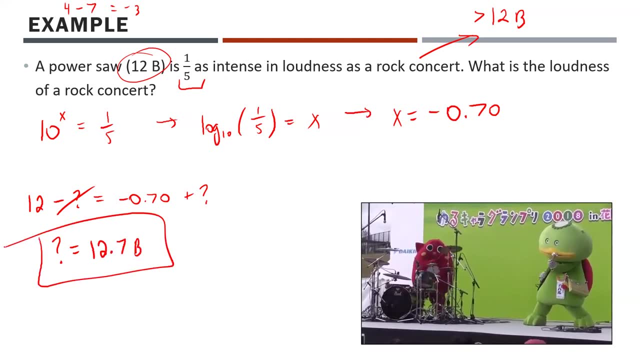 rid of negative 0.70,. I'd have to add that on both sides. Long story short, you're going to get question mark equals 12.7 bells. That would be the loudness of the rock concert. So if you have a 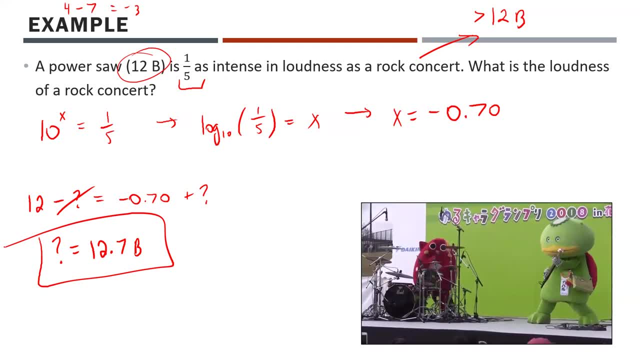 rock concert, right, So the rock concert has a higher loudness than the power saw. Not a big surprise, right? Anyway, moving on, I think we're almost done. actually, if it's going to let me move on, There we go, There we go, All right. So here's a chemistry example: The pH of a solution. 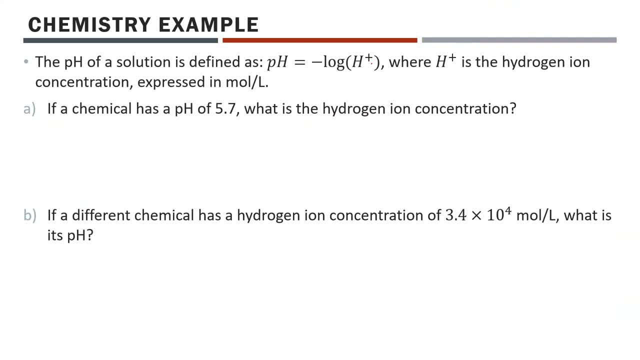 is defined as pH equals negative log H positive. So it's pretty weird. So what we're doing here is we're comparing the pH to its actual component, the thing that actually makes a pH right. So H positive is the hydrogen ion concentration expressed in moles per liter, If you've not taken 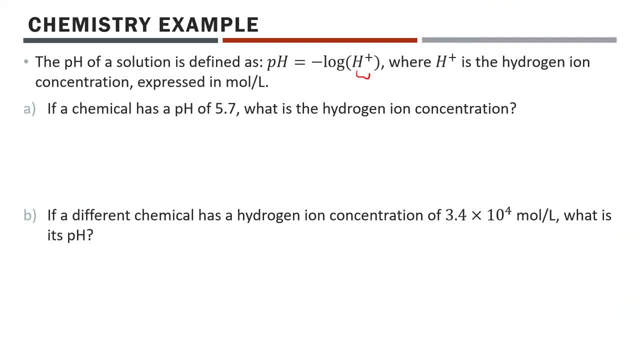 chemistry, don't sweat this too much. Just try to look beyond what it's asking. Just try to calculate the numbers. I'm not going to require you, of course, to know any chemistry in this. So let's say, a chemical has a pH of 5.7, right, So we know the pH 5.7.. What is the hydrogen ion? 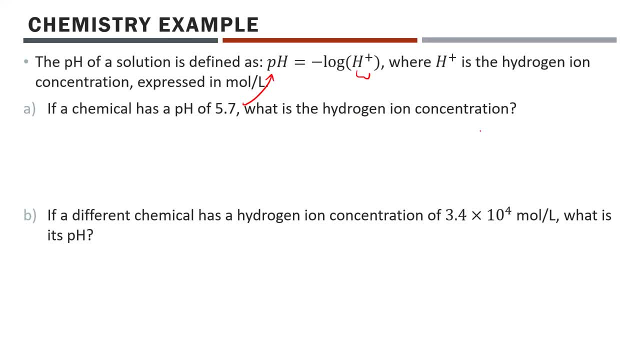 concentration. There's no tricks on this one. We're not dealing with intensity differences. We don't have to use that whole difference, And then we're going to use the pH of 5.7.. So we're going to use the pH of 5.7.. So we're going to take it to the power of that thing. We can just throw this right. 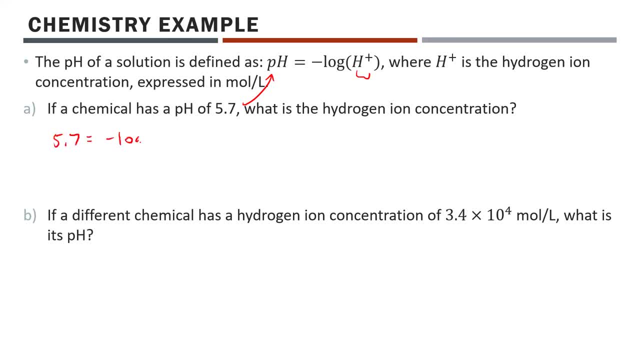 in. So we can say: 5.7 equals negative. log of H positive. Now we like to. of course, if we have to solve a log, we have to solve what's inside the log. We'd like to turn this into an exponential. 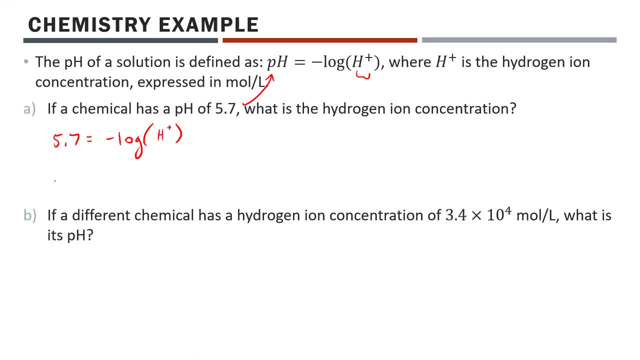 function, but we have to get the logarithm by itself first. So I'm going to move the negative to the other side. Negative 5.7 equals positive log of H plus. Now I'm going to turn this into an exponential function. Start with your base, Because it didn't list a base here. 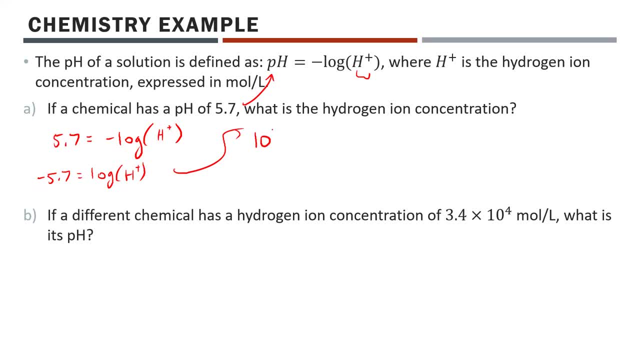 you have to assume it's 10.. So base to the power of the answer. So the power of negative 5.7 equals the thing that was in the log. So H positive. And boom, there, it is right there. You can just throw that straight in your calculator: 10 to the power of negative 5.7.. 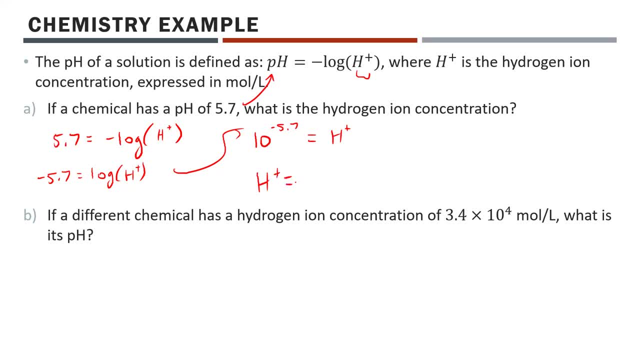 It's going to give you kind of a gross number here. H positive equals, we'll just say to- I was going to say to two decimal places. but what's funny here is, either way it's going to round right up. This is going to round right up to 2.0.. And then it says E negative. 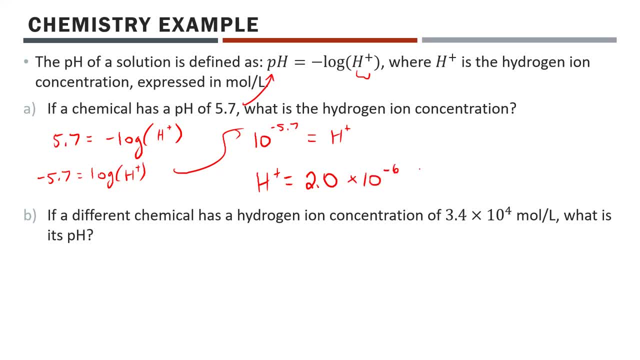 6 means times 10 to the negative 6.. Oh, and then the units, of course. moles per liter. If the question gives you units, try to respect that. That's all I've got to say, right? Next one: If a different chemical has a hydrogen ion concentration of 3.4 times 10 to the 4 moles, 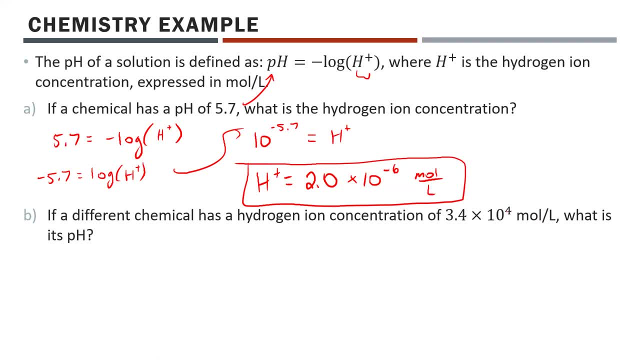 per liter. what is its pH? Oh, interesting, That's quite a high concentration there. Well, let's find out. So if a different chemical has a hydrogen ion concentration of that, let's see, We just have to throw that in there. So pH equals negative log. 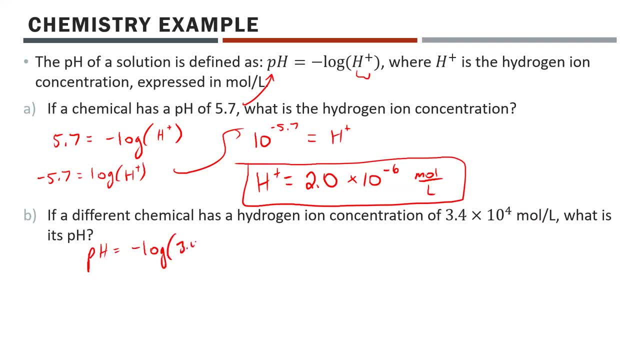 of that hydrogen ion concentration, which is 3.4 times 10 to the 4.. Just throw that straight in your calculator: Negative log 3.4 times 10 to the 4. It's probably going to give us a really low pH, Yeah, really low pH. So this is kind of a broken. 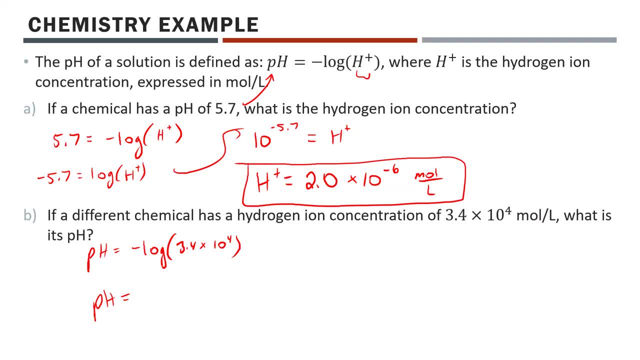 question. I don't like this one at all. The pH of this following this formula- and this is serious, we didn't do any math wrong here- is negative 4.5.. Wow, That's like a hyper pH right there. 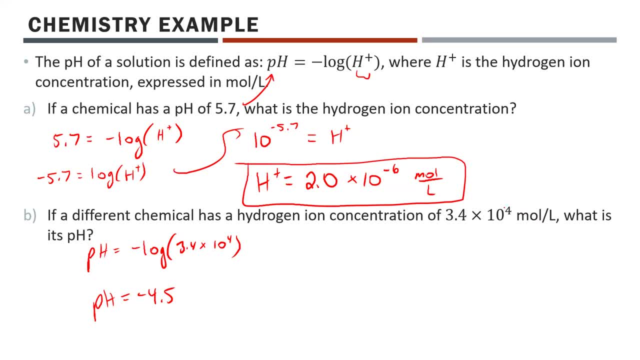 That's insane. This question- actually this probably- is actually a typo. What if it's 10 to the negative 4?? Maybe we'll even just try that, just so we get something a little more reasonable here. For those of you who have taken chemistry, you know pH is usually just between 0. 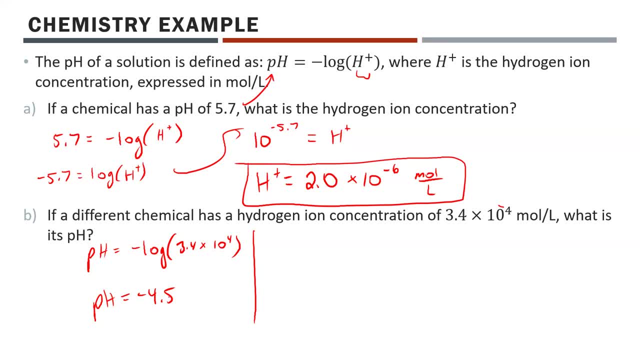 and 14.. Having a negative pH? that'd be pretty wild, right. Let's try something else in this one. Let's make that 10 to the negative 4.. That might be just a typo here. So pH equals negative log of 3.4 times 10 to the negative 4.. Let's do that one a little bit better. I think I'm 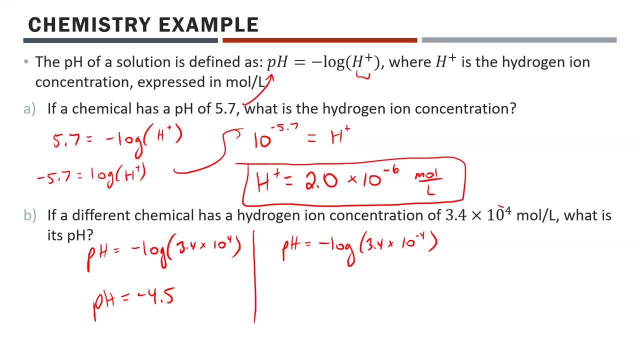 going to correct that Future years, because that definitely is going to make that a little bit better. Anyway, typing that in my calculator now: Oh yeah, much better. We'll just do it to two decimal places. pH equals 3.. That'll round up to 3.5.. So 3.5 would be our pH there. That's a little bit. 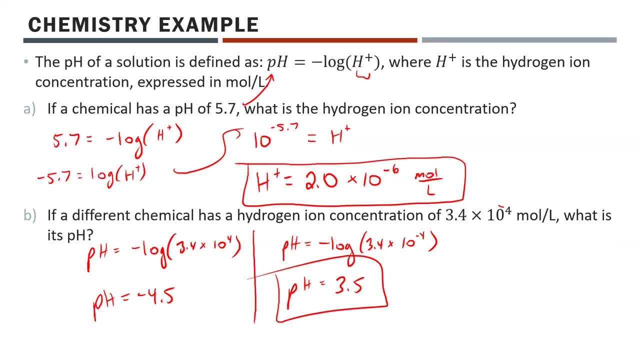 more comfortable than having a negative pH. Yeah, I apologize about that. You know what I'll own up to, that. I'll make sure I change that in our note packages going forward. So 2022, you guys are the last group to ever have seen something that garbage. But anyway, moving on. 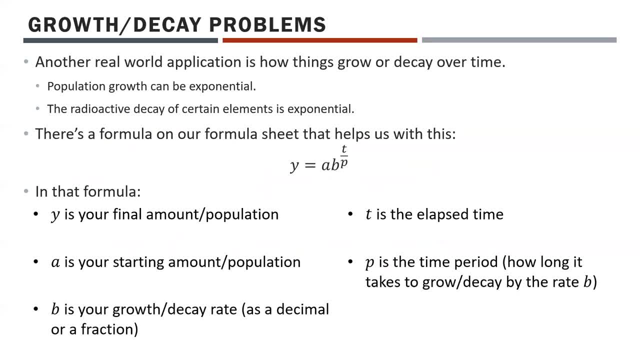 Believe it or not. we're not quite done yet. We have a little bit more that we have to cover here. Growth and decay problems are a really, really big application of this. Now it's more an application with exponential functions, of course, But believe me, this is also something that comes. 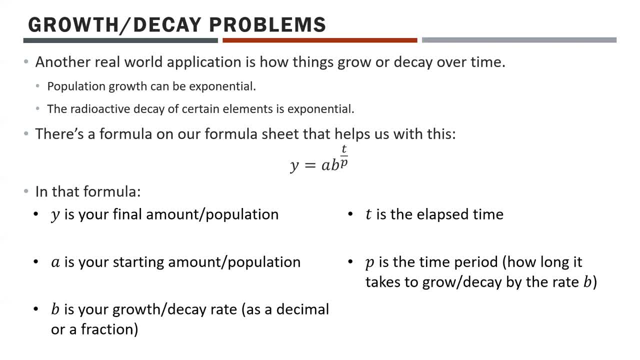 around with logarithms as well. So another real world application is how things grow or decay over time. So a couple examples of this would be population growth. That can be exponential, especially if it's like a virus or something. Radioactive decay of certain elements is exponential. 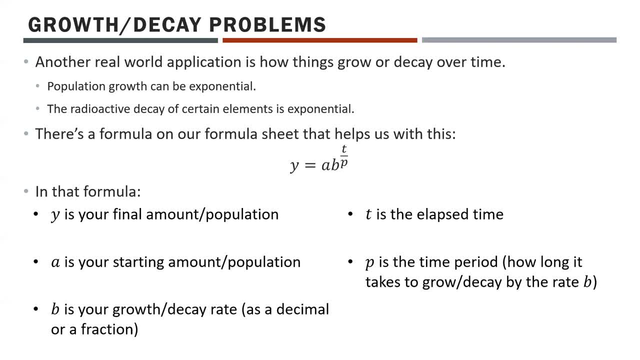 So that would be something you'd see in a lot of other things. So that's a little bit more of a something you'd see in physics 30.. There is a formula on our formula sheet- lucky you guys- that actually helps us with this- Straight from your formula sheet. it says: y equals a times b to. 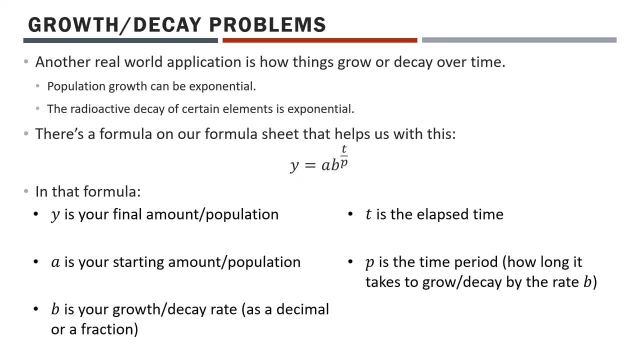 the power of t over p. It is unfortunately your job to understand what each of these letters mean, But if we break it down from what we know, it shouldn't be too terribly bad. Y is your final amount or population. A is your starting amount, right When we were first? 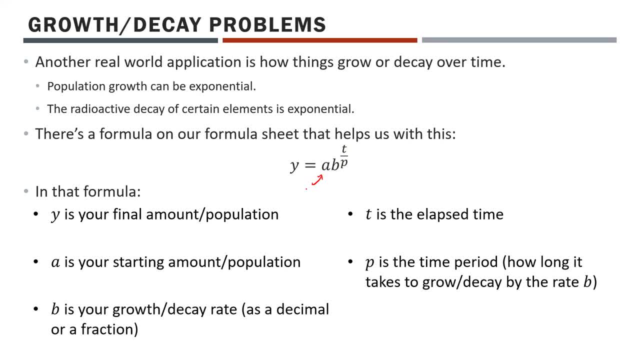 learning about exponential functions. at the start of this chapter we were learning about exponential functions. We were talking about how a in an exponential function is your y-intercept- That's your starting amount, right? B is your growth or decay rate as a decimal or as a fraction. Remember if b is bigger. 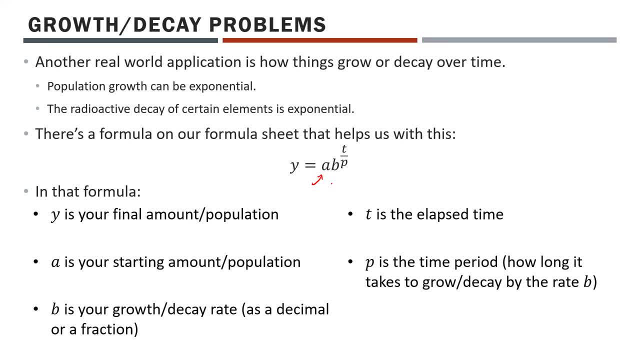 than one, you're growing. If b is between zero and one, you're decaying. right T is the elapsed time, So it's how much time has passed since this growth or decay thing was watched. And then p is the time. 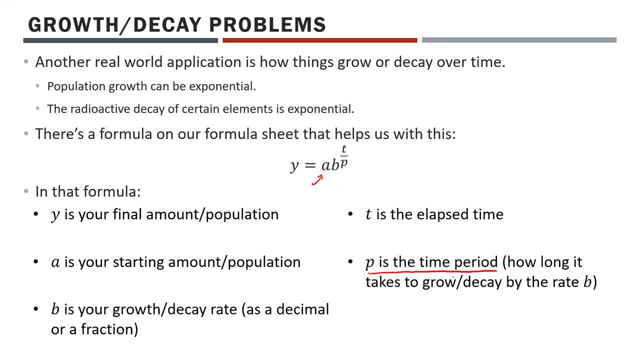 period, which is one of the fancier things here, That's just how long it takes for it to grow or decay by the rate b. So if I told you, oh, b is the time period, which is one of the fancier things here. 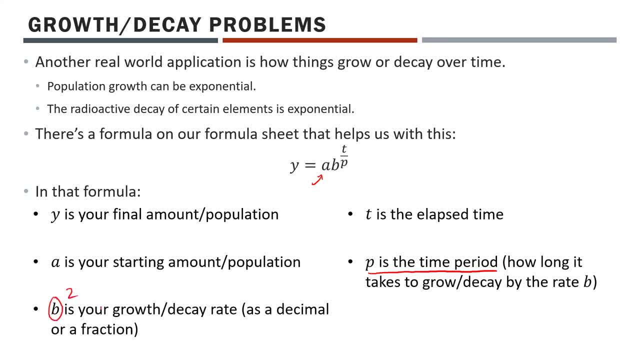 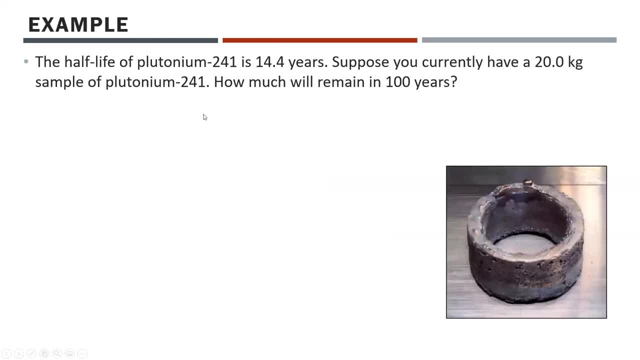 it doubles, So b would be two. If it doubles every five years, well then p is five years, So it'd be. you know, p would be the denominator of the exponent there. Anyway, let's see an example Hitting out the big guns here. first We're going to look at a physics 30 half-life question. 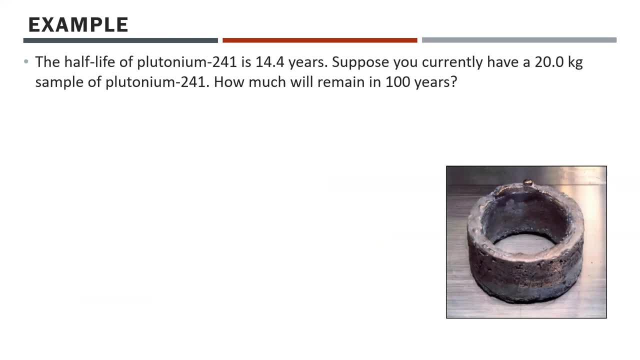 The half-life of plutonium-241 is 14.4 years. Suppose you currently have a 20.0 kilogram sample of plutonium-241.. How much will remain in 100 years, In case you're not aware, with half-life? 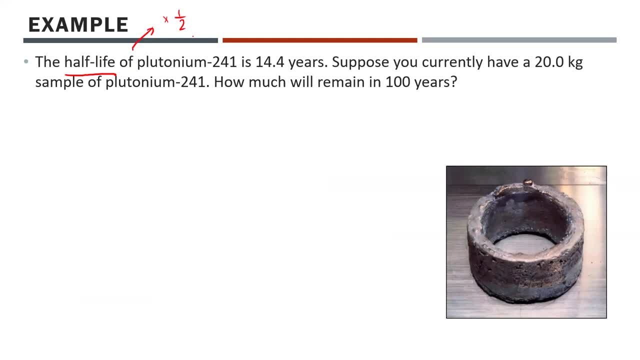 half-life just means we're multiplying by one half, in this case every 14.4 years. Let's set this up: Y equals a times b to the power of t over p. That's our formula. We want to find how much will remain. That's going to be our y equals. figure out how much you were starting. 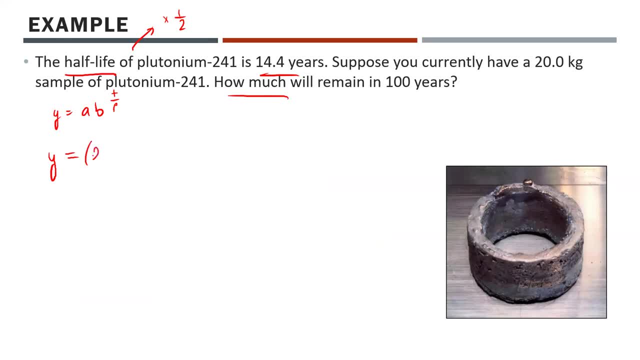 with. That's your a value. You currently have 20.0 kilograms, So I'm just going to say 20.. The half-life: that means we're multiplying by half each time, So that's going to be our b value. 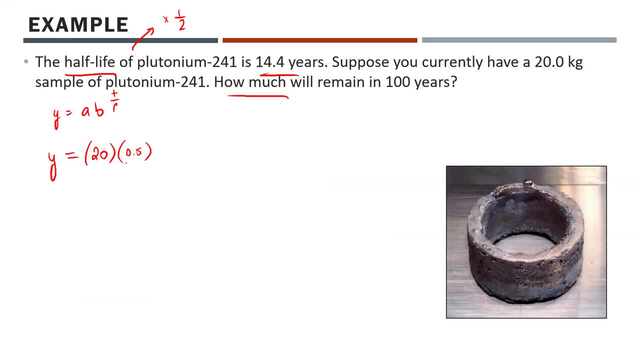 I like using 0.5.. You can use literally one half. I'm going to fix that 0.5, though. There we go. You can literally use 1 over 2 if you want, but I prefer the decimal. It's just a matter of. 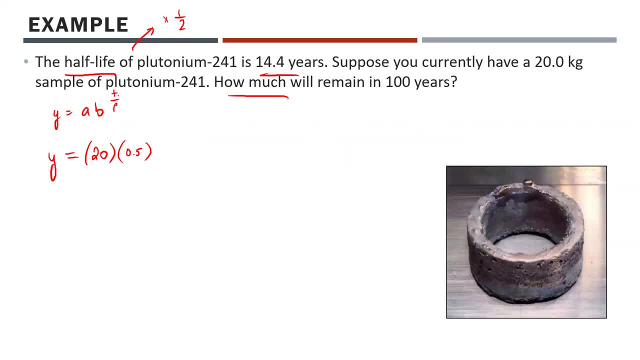 preference To the power of t over p. Well, t is the elapsed time. We were told. this is going to go for 100 years. So 100 over p is the time period. That's how long it takes to be cut in half. Well, 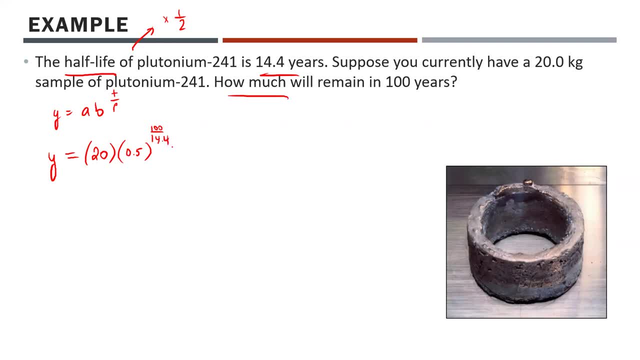 that'd be 14.4.. Just a matter of throwing that in your calculator. at this point I could have made this question a lot harder and told you how much like was left, and told you to like find how many years were passing. But you know what? I guess? 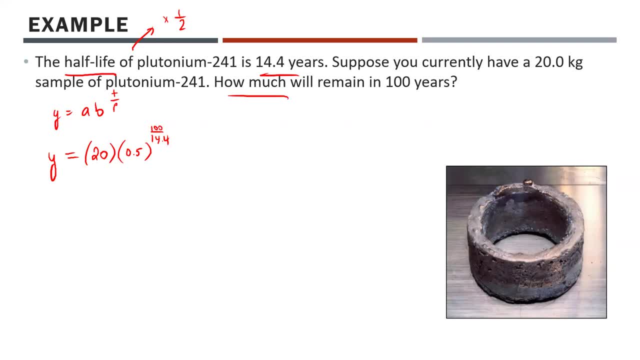 I was nice to you. So, anyway, throw that in your calculator. 20 times 0.5 to the power of this- really, You'll want to put that in brackets when you put in your calculator, of course- To the power of 100 divided by 14.4.. This is going to give us y equals 0.16. And that, yeah, that's. 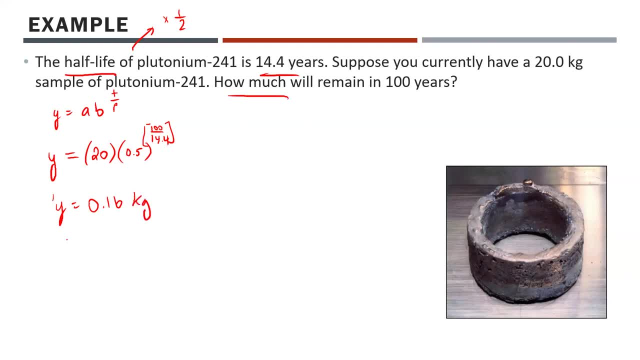 not a typo, That is, that is correct. 0.16 kilograms. You're not going to have very much left over after 100 years, right? So most of it's gone at that point. After 14.4 years, you'd only. 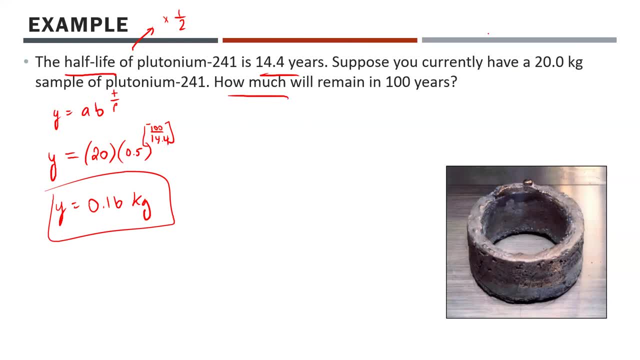 have 10 kilograms left After another 14.4 years. you only have 5 kilograms left After a full 100 years past. you don't have all that much left right? It's all. it's all gone away, right. 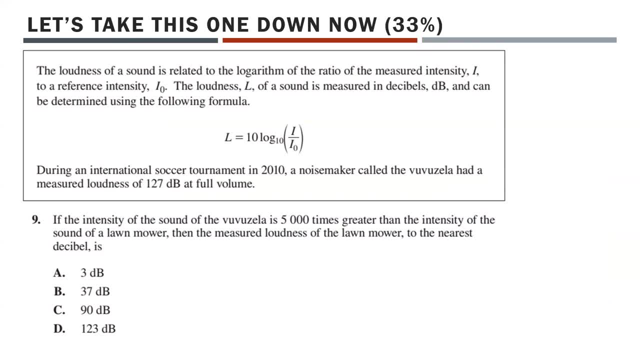 Now grand finale here. Like I said, everything's coming full circle And I'm going to prove it to you here. I want you guys to give this question a try. This is the same one we looked at at the start. Again, 33% correct rate. I want you to use what we've talked about. 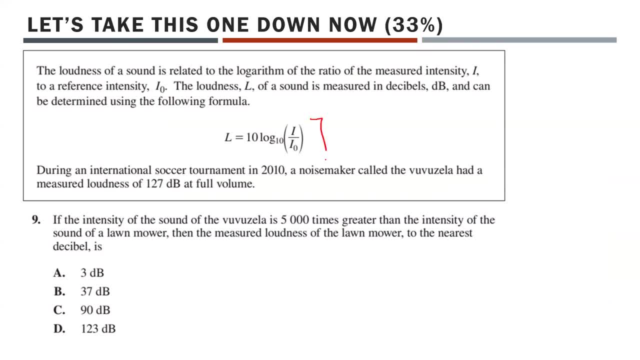 Today, At the very beginning of the lesson, when I showed you this, I say the formula they give to you here pretty much baloney There's. there is a way you can use it. I just don't really see it as. 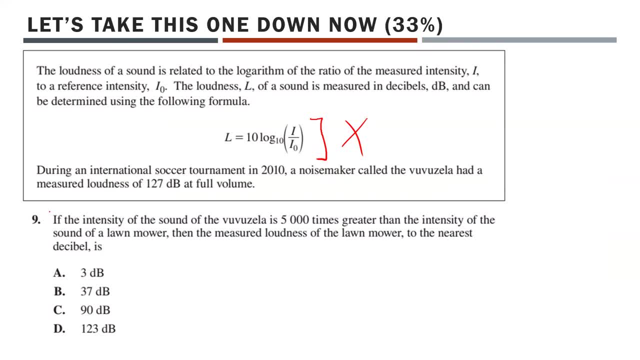 being a very easy way at all, So I'll just read the actual question part to you. You'll want to read the box up here too, Especially this: the fact that it's 127 decibels If the intensity of the sound of a Vuvuzela is 5,000 times greater than the intensity of the sound of a lawnmower. 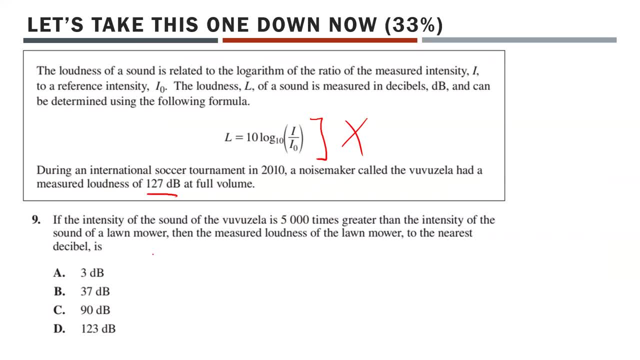 then the measured loudness of the lawnmower to the nearest decibel is going to be 5,000 times greater than the intensity of the sound of a lawnmower. So I'm going to give you guys an honest shot here. I'm going to give you guys an honest shot here. 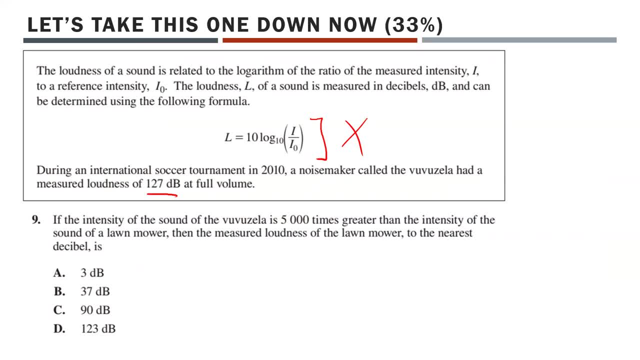 So I'm hoping you actually give this an honest shot. Let's see if you were able to get this one right. If you have a really good intuitive understanding of how the decibel system works, you could actually just guess and check this one and you'd be just fine. Some actual reason could. 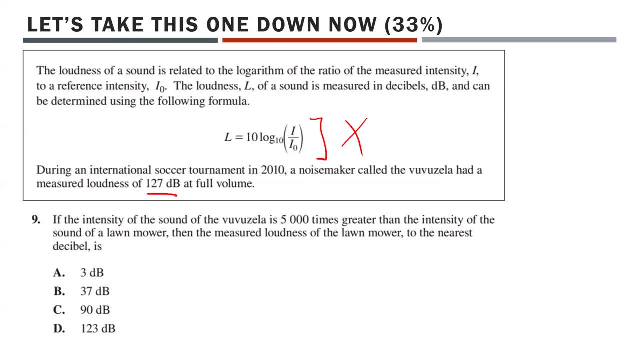 actually solve you through this. But in other diplomas I've seen they've been a little bit more sneaky with this. So we do need to know the proper way. Remember the rule is we want to find the difference between the intensity of the sound of a lawnmower and the intensity of the sound of a. 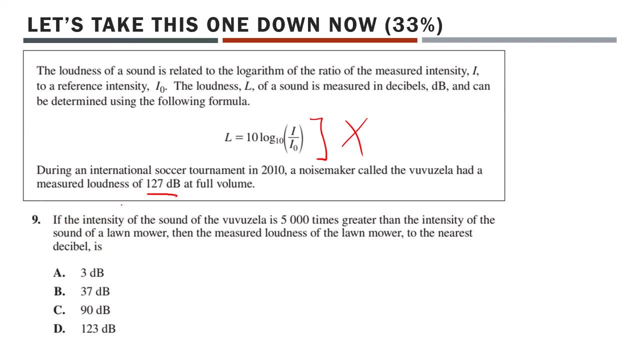 loudness. That is what we take to a power to give us our difference in intensity as, like a times factor, We were given that times factor. at the end here It's 5,000 times greater. We're going to have to start there and work backwards like we did on those later examples. 10 to the power of 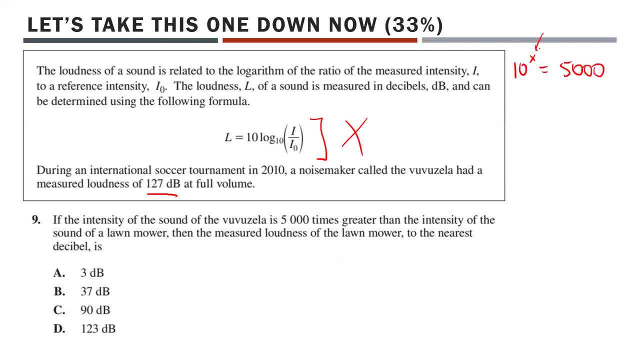 something equals 5,000.. That something represents our difference. That's the difference between our loudnesses. I guess it would be in bells, Remember that'd be 12.7 bells instead. So to find that x, we just need to turn this into a logarithm Log, base 10, because we had the base of. 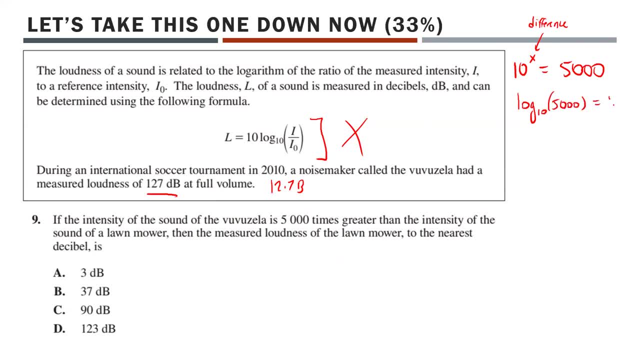 the exponent was 10 of our answer, which is 5,000 equals x. Throw that in your calculator Log base: 10 of 5,000.. That gives me roughly 3.7.. So x is 3.70.. Okay, Hopefully you're with me. so far, Remember. 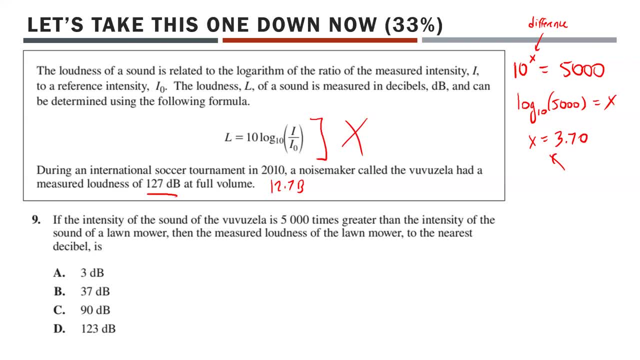 that number there, 3.70, that represents our difference. The vuvuzela at 12.7 bells, like forget decibels, always turn it to bells. 12.7 bells is going to be the bigger number here, So we're going to have 12.7 minus the lawnmower. 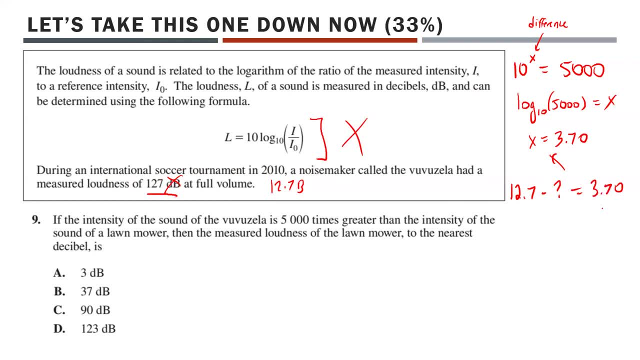 I'll just call it. question mark equals 3.70.. To solve for the question mark, just a bit of basic algebra. add the question mark over subtract 3.7, bingo, bango, bongo, you're going to get. 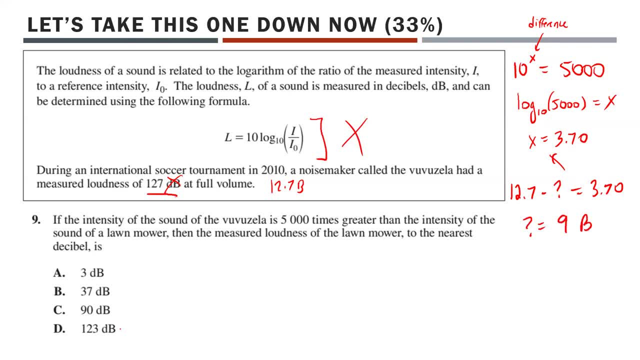 question mark equals nine, and that's bells. Back to decibels, though, right. So nine bells is great for doing our math. For actual communication, we use decibels to express loudness. That's 90 decibels. Boom, You got that. You're already ahead of, I guess, 67% of Albertans. Holy smokes. 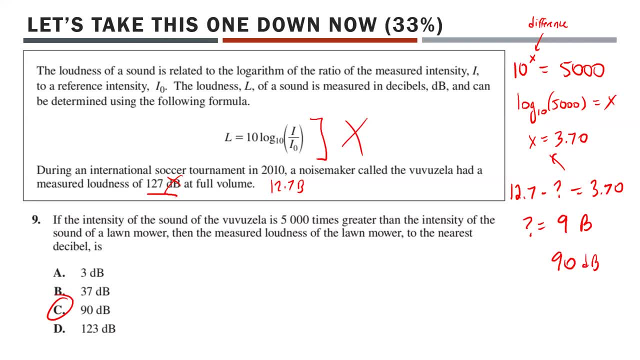 right Again. I think the reason why this question had such a low success rate is mostly because this formula always throws people through a loop Anytime you see difference in intensities like 5,000 times greater or whatever. I don't bother with this If you want to snoop around with it. 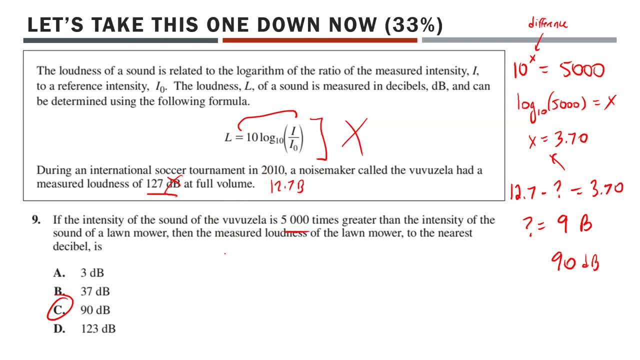 and see if you can figure out a way to make some sense out of it. you're more than welcome to Personally. like it doesn't define me Measured intensity versus reference intensity. we weren't even given all that many numbers. I don't really see much use in this formula personally, but that's just my opinion Anyway. 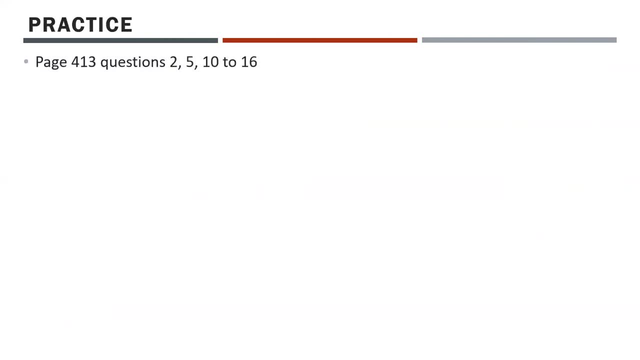 for practice. here's some practice questions. Very wise idea to give these a shot. If you need any help, please let me know. 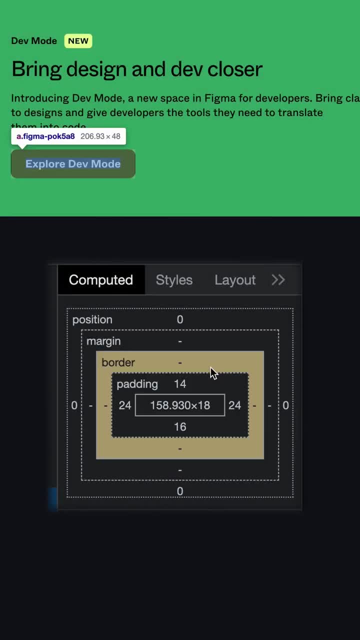 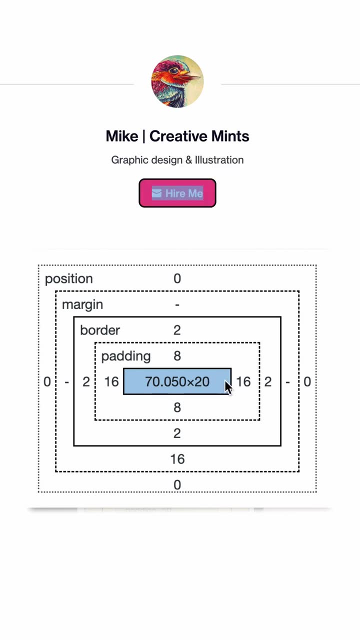 In web development, we essentially use the box model to tell the browser how it should display the content on our screen and how it should space all the elements on our web page. The innermost part of the box is the content. That's your text, that's your image. Next up, we have padding, which 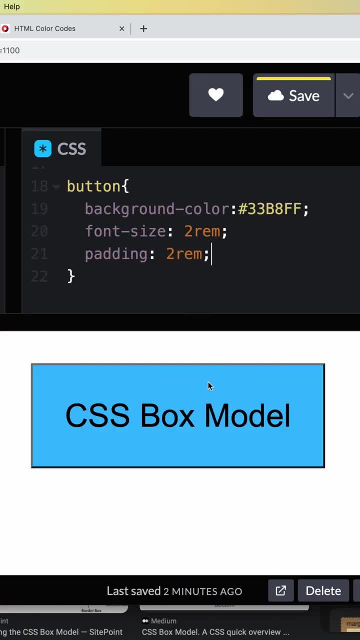 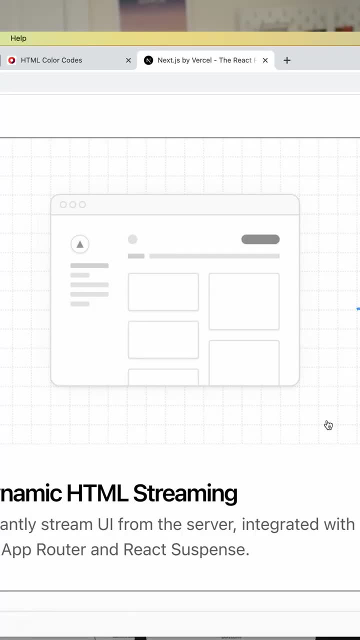 I like to imagine it as giving extra breathing room to your content. We have border which you can add on the outer side of the padding, and you can use that to style up secondary buttons if you want, or create some fun grids. Martin represents the space outside of the element and this is where 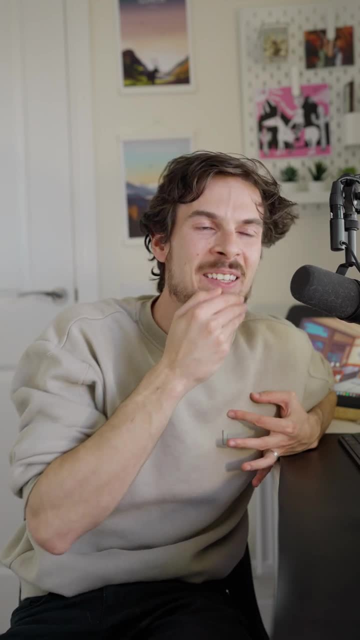 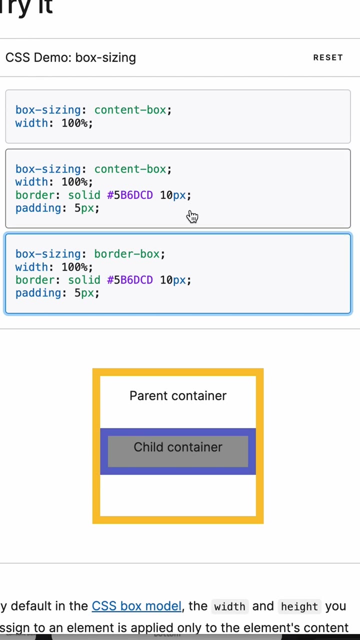 it gets funny with padding and margin and all of these different things. If you have it on content box, your element essentially is going to grow in size when you're increasing the padding. but if, when you have it in border box, that padding is always going to be on the inside, not changing the 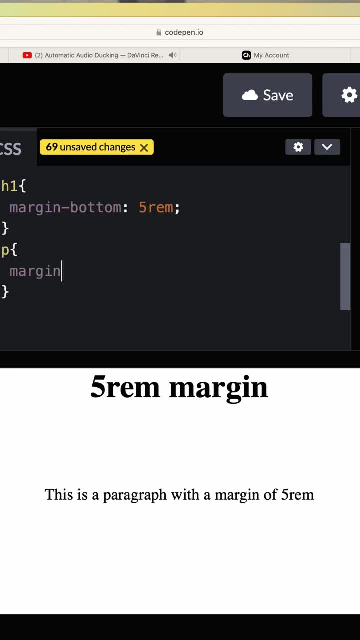 size of your element. Now also be aware of something called margin collapse. If I have an element that has a margin of 5 and another element that has a margin of 6, the space in between the elements is going to be margin of 6, whereas with padding, space in between here is going to be 10.. So yeah, anyway.